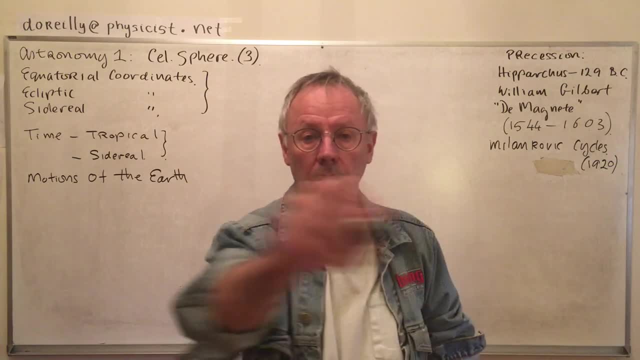 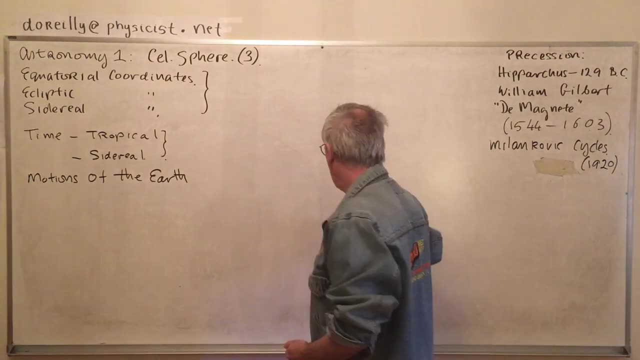 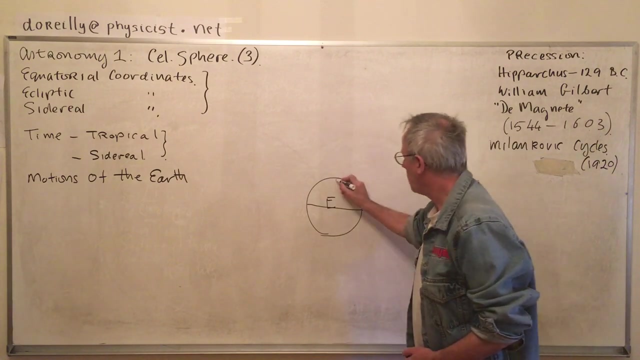 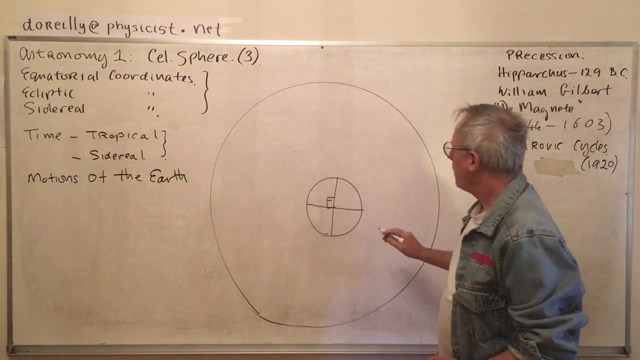 Right ascension. it's like celestial longitude Declination, celestial latitude. Now where is it measured from? as I discussed, We put the Earth with its equator and axis inside the celestial sphere, And the celestial sphere contains a projection. 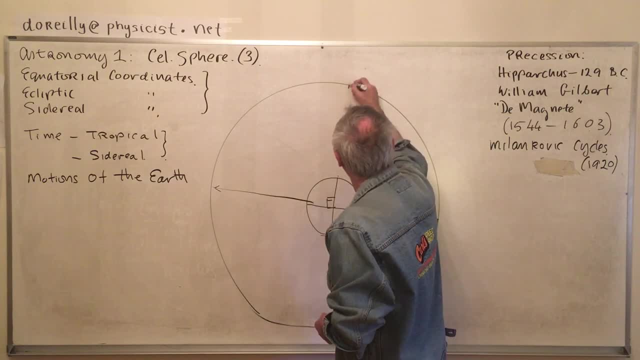 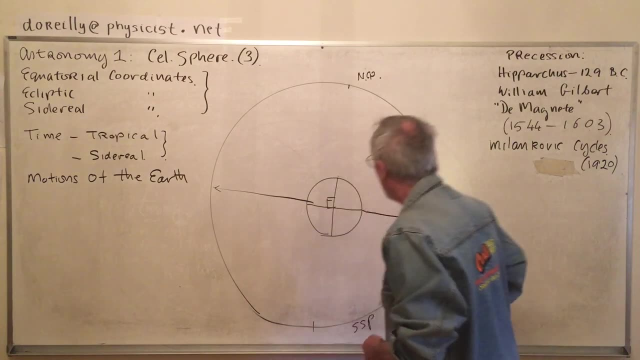 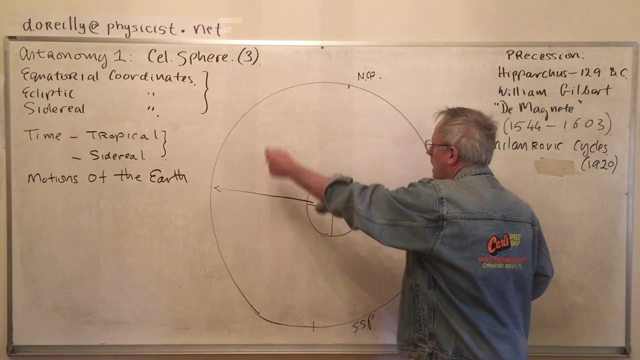 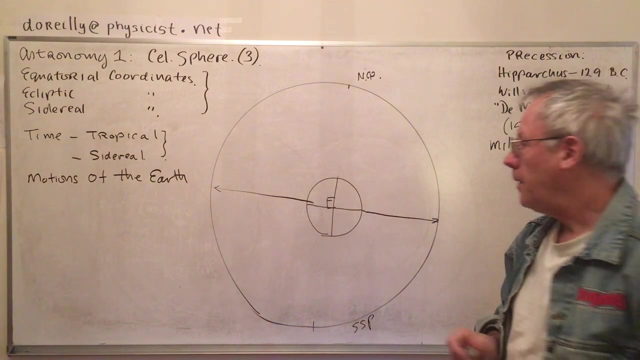 Of the Earth's equator and a projection making the north celestial pole and the south celestial pole as points on the equator. Now, as the Earth revolves, this celestial sphere appears to revolve to us, but we're actually revolving. Now we're doing more than revolving, and that's what complicates things. 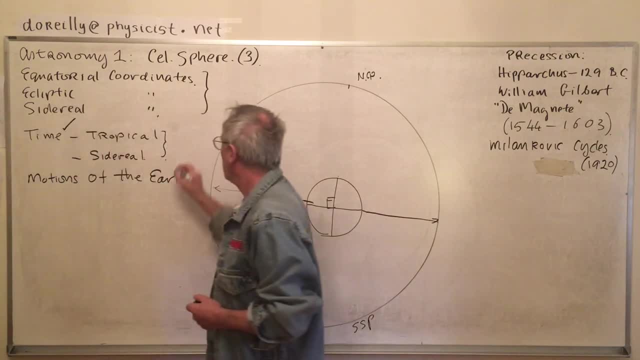 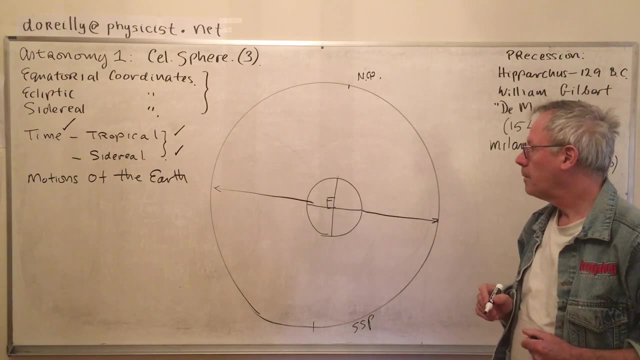 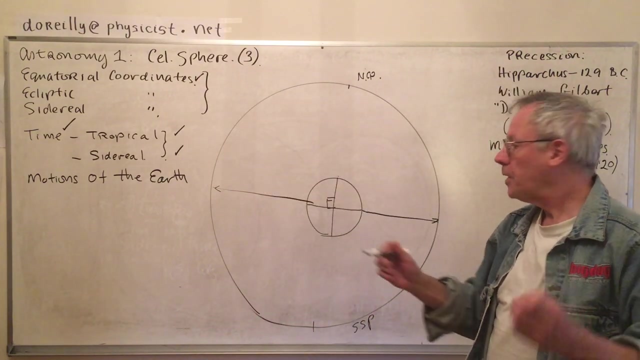 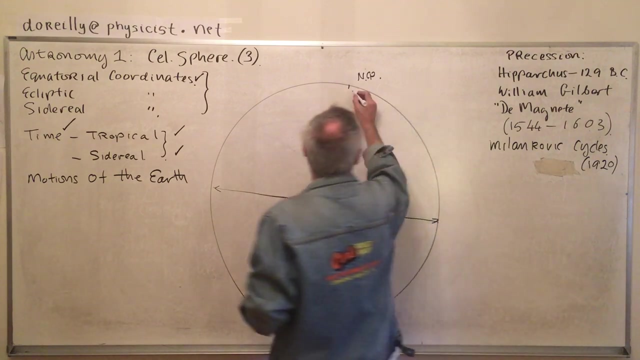 When we want to figure out time In terms of the Sun as compared to the fixed stars, it gets complicated and different. Not only that, when we want to make coordinates, it gets complicated and difficult because nothing is fixed. Now we can base our coordinate system on the equator, the celestial equator, and then we get celestial, let's say, declination. 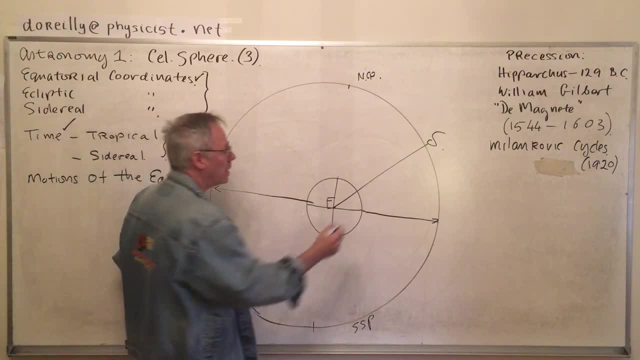 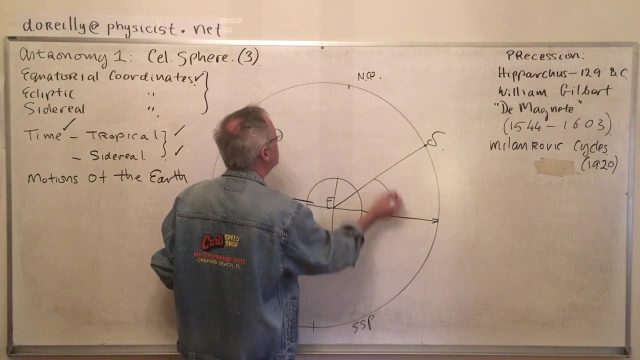 Right And the star will have a certain altitude in the equator, Altitude in the night sky, altitude above the celestial equator, and that goes from 0 to 90 in the case of declination and negative 90 south of the celestial equator. 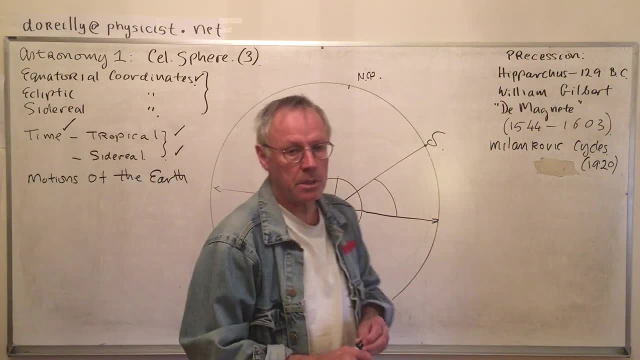 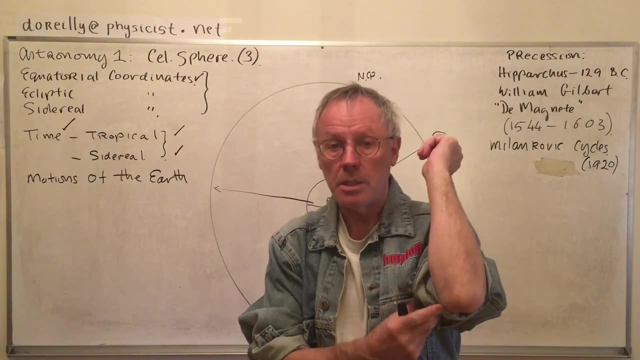 We discussed this already. Now I didn't get around to doing examples of showing you where stars might be, but you know you can get that on the web. I'm just doing a basic for-interest introduction to this because I'm not really an astronomer. 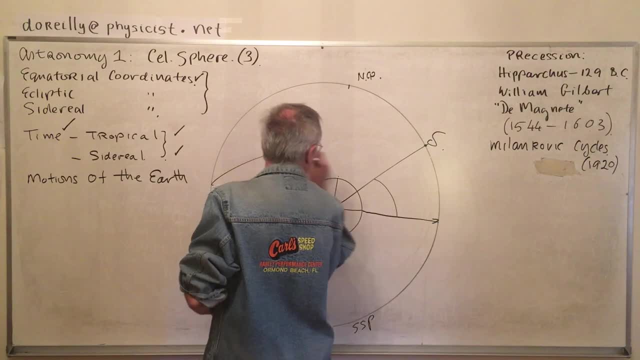 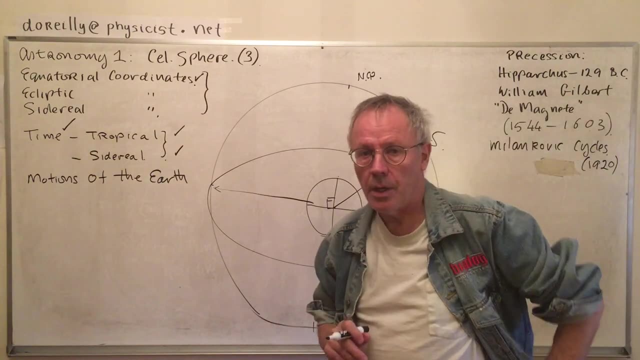 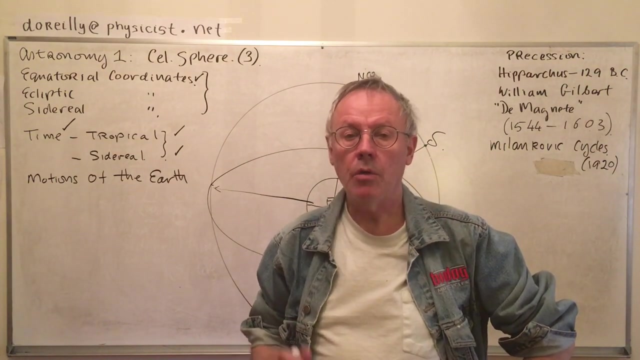 All right, then the next thing: right ascension. Well, the right ascension works. like longitude. Well, we need a prime meridian for our longitude on the Earth. We choose the meridian or great circle that goes through Greenwich, not Greenwich. Greenwich in London, the Royal Observatory in Greenwich, down there on the Thames in London. 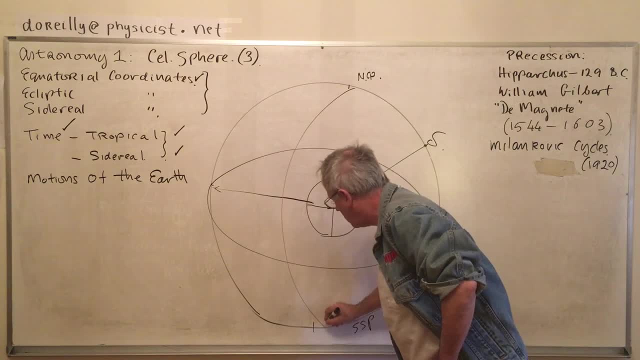 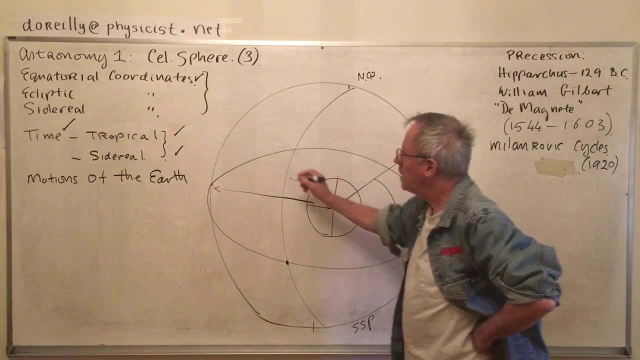 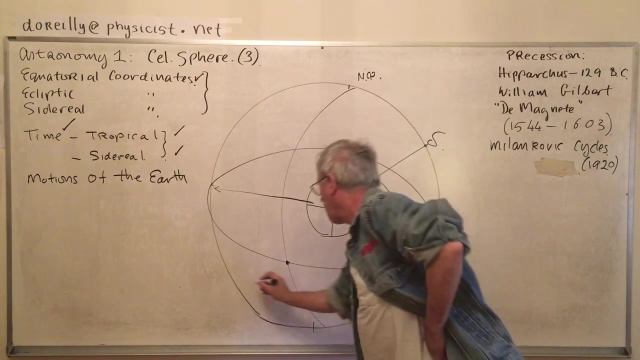 That's called the prime meridian, and it's 0 degrees longitude in the case of the Earth. Now, in the case of our celestial coordinates, the equatorial ones, the beginning of our right ascension is going to be here, Where 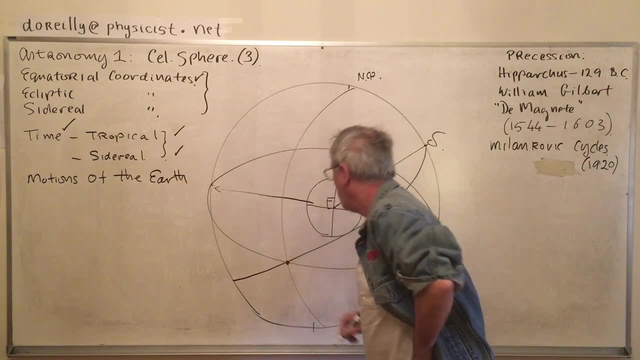 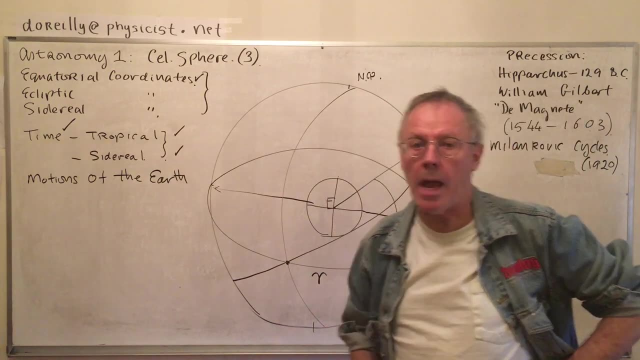 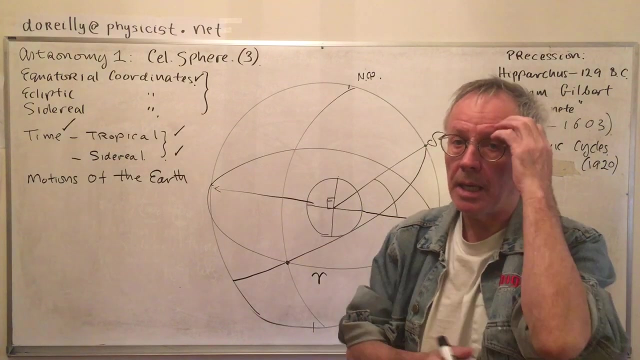 Where the ecliptic cuts the celestial equator, It's called the Virgo Equinox. That's the symbol of a ram, The first point in Aries. What does that mean? Where Aries as a constellation begins. I'll talk about that as a while too. 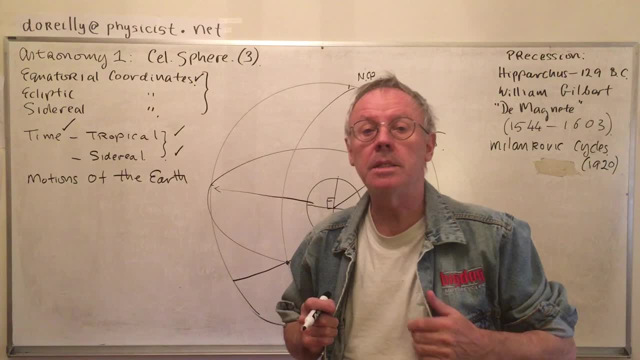 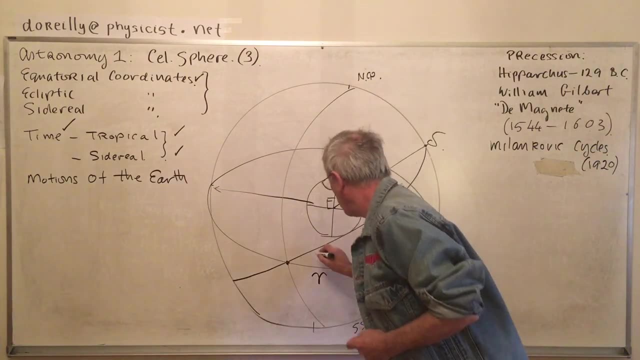 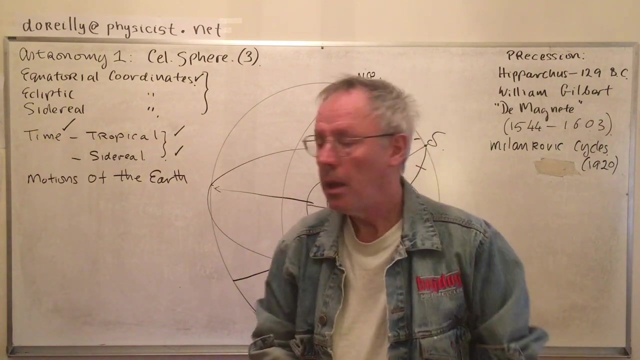 You don't really need those stars up there to designate those constellations. They're just boxes right With a certain angle. Now you can measure the angle in degrees All the way around from 0 to 24.. Did I do that right? 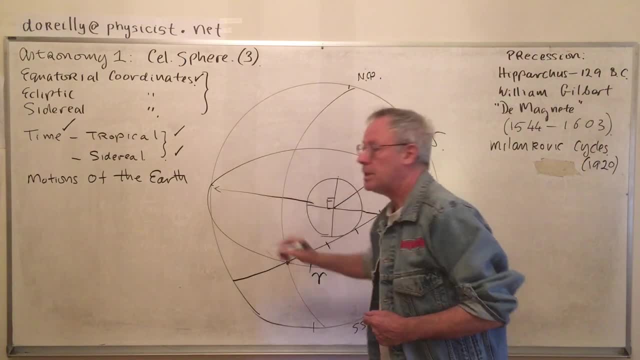 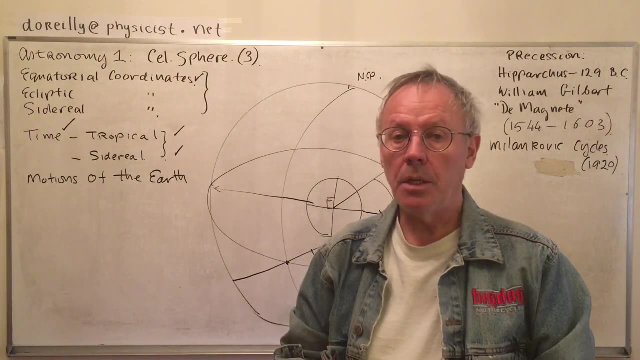 No, I meant to do it this way All the way around on the celestial equator, Or you can measure. that's what I do, actually. I use degrees, But astronomers like to use hours, Because another way of looking at declination is that. 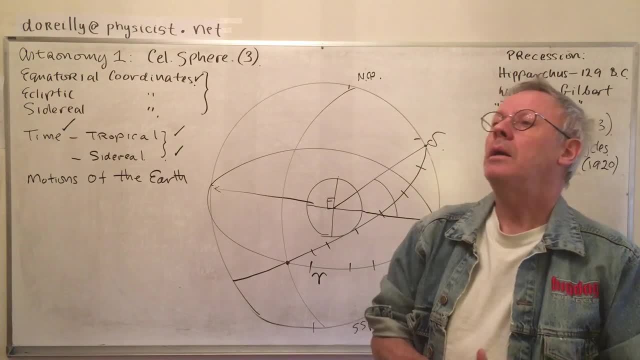 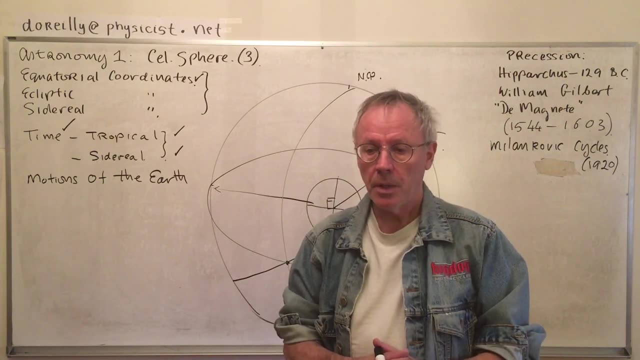 or the 21st of March, is it? I forget. The declination is the time behind the number of hours behind the sun, The time behind the sun. So a star that's two hours behind the sun will rise two hours after the sun rises. 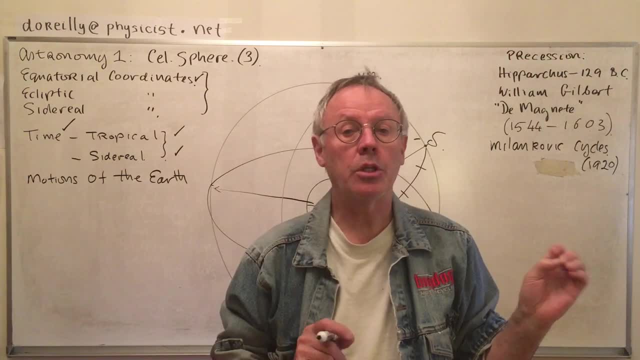 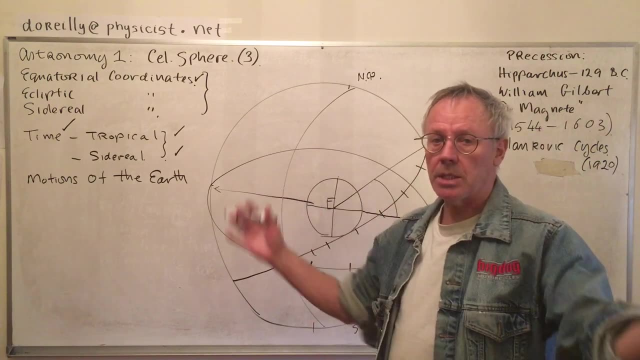 That will be sorry. that would be a star with two hours right ascension And so on. It kind of makes things easy if you're an astronomer, Now okay. so all this stuff gets extremely complicated due to the motions of the Earth. 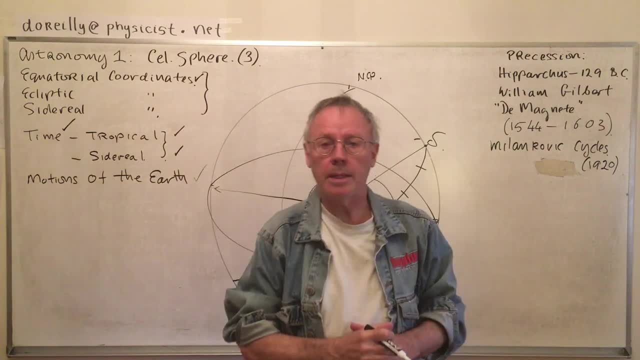 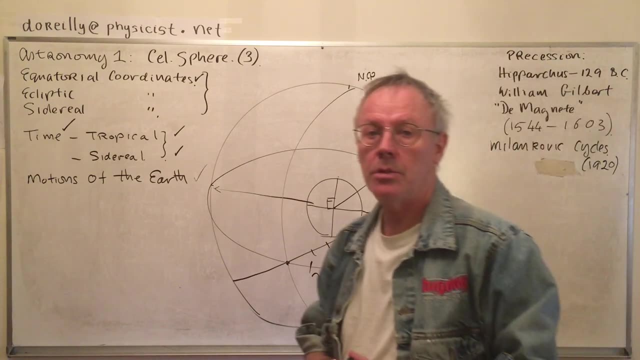 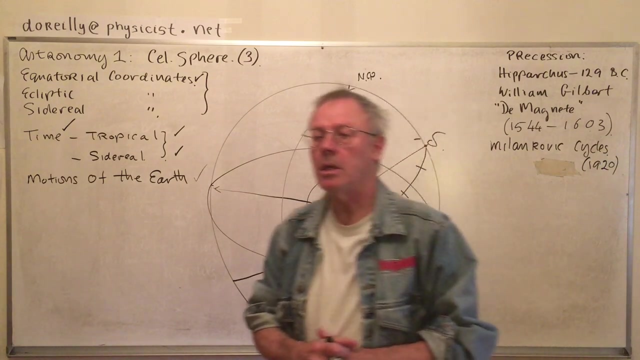 So I just want to very quickly talk about some other coordinate systems. All right, I want to talk about the coordinate systems that I would like to use: Sidereal, okay, Sidereal. Well, people are. I think that astronomers could well be in the process of renegotiating. 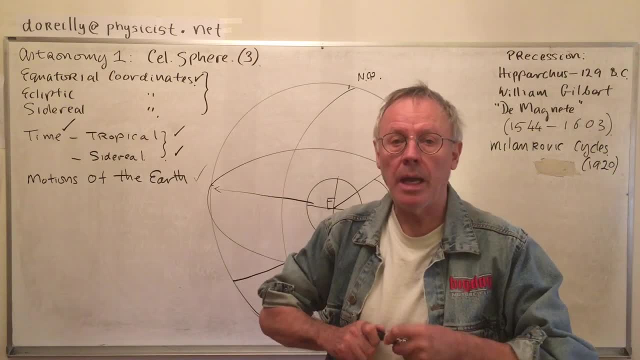 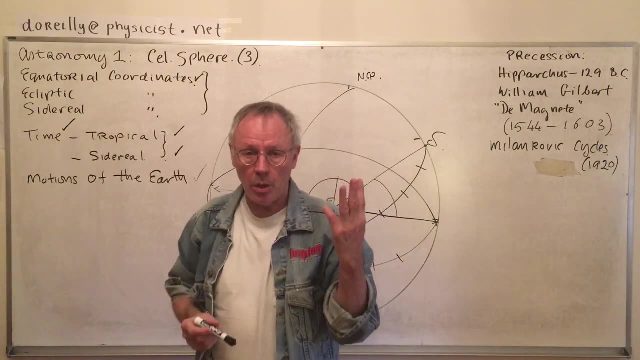 what coordinates they're going to use. So first of all, I want to see show you where things begin to get complicated. So equatorial, ecliptic and sidereal are three types of coordinates, But there are many others. There are sun-centered coordinates, There are moon-centered coordinates, There's altitude and azimuth coordinates, and so on and so forth. But as the night sky is moving all the time and it has complicated motions, one coordinate system will always, you know, have some benefits over another. 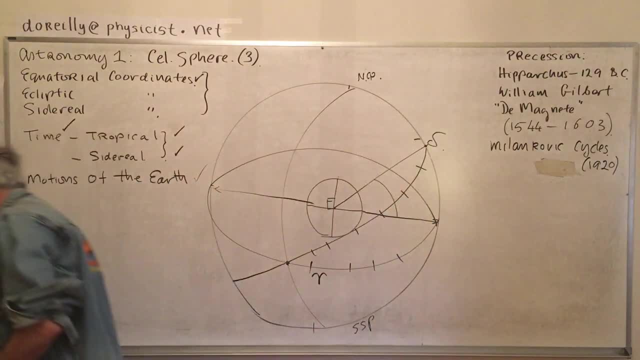 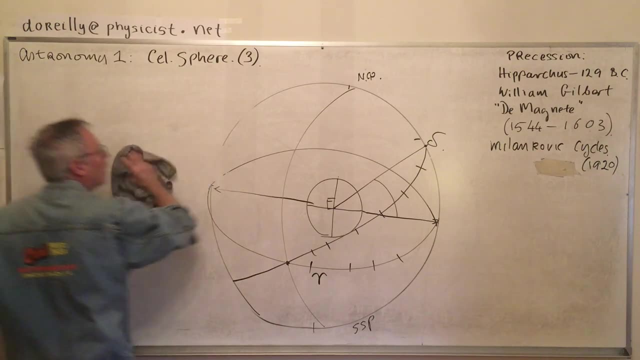 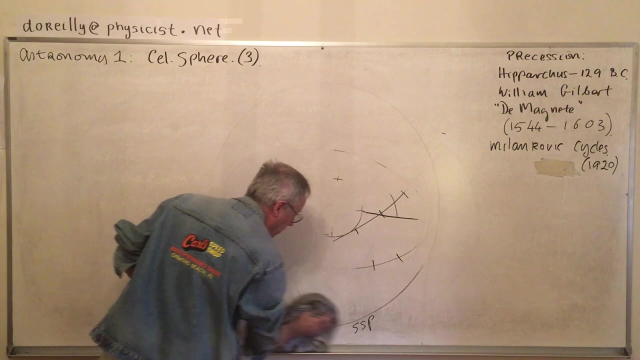 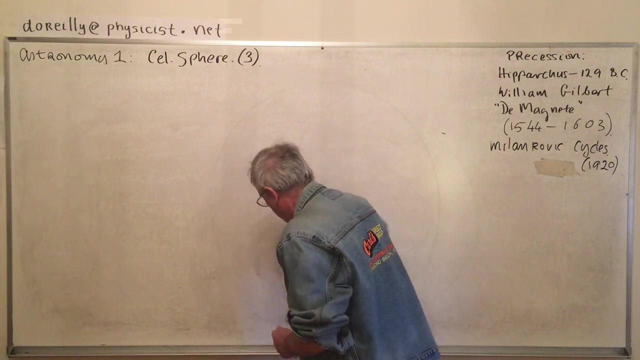 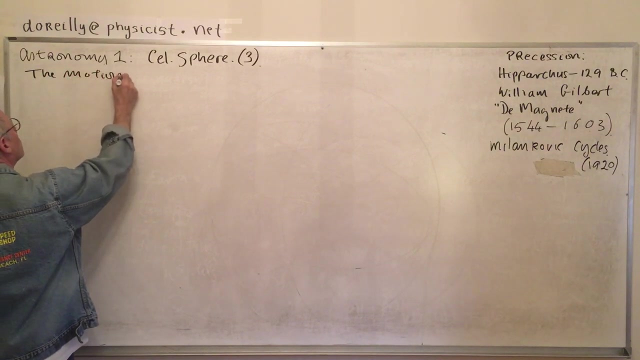 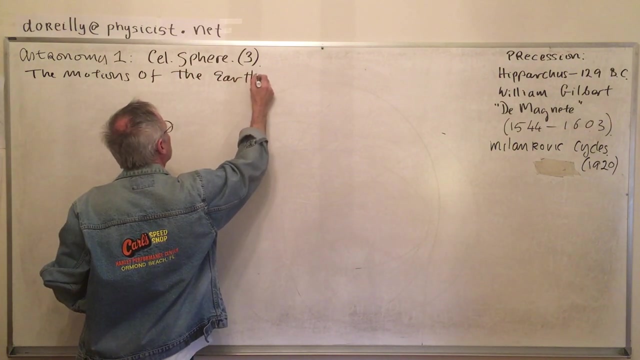 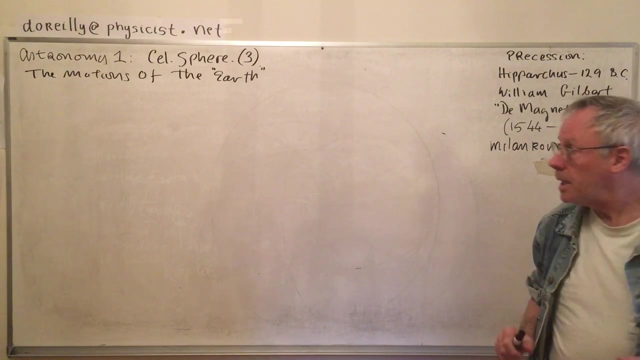 depending on what your requirements are. That's a long story. Now I'm going to list the motions of the Earth first, And then I will discuss them. Well, it's really the Earth-Moon system, Because the Earth-Moon system has a center of mass which is called the Barycenter. 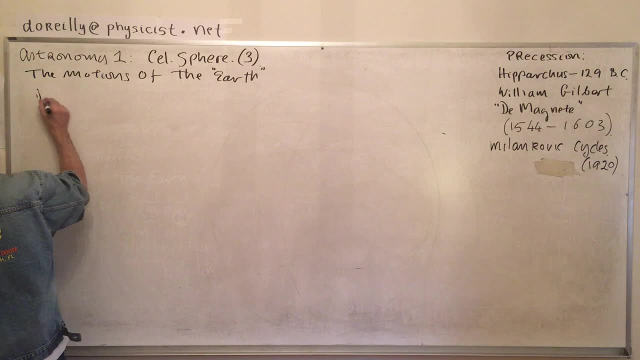 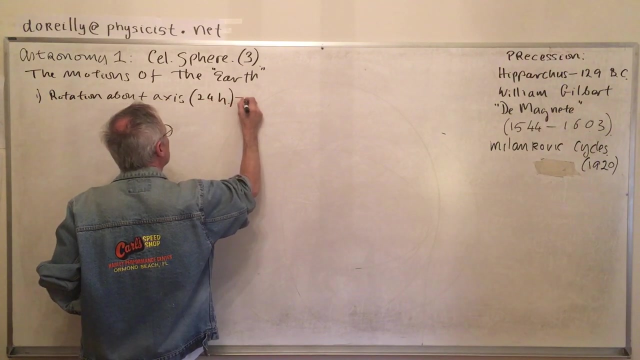 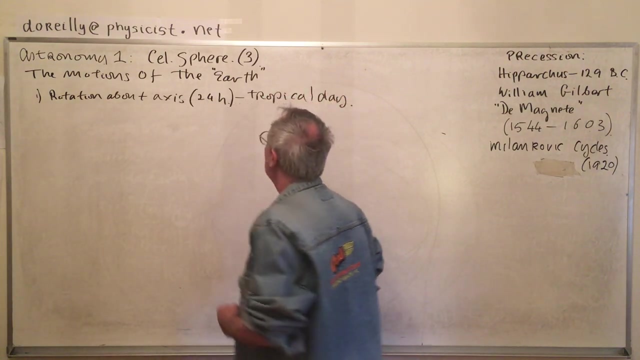 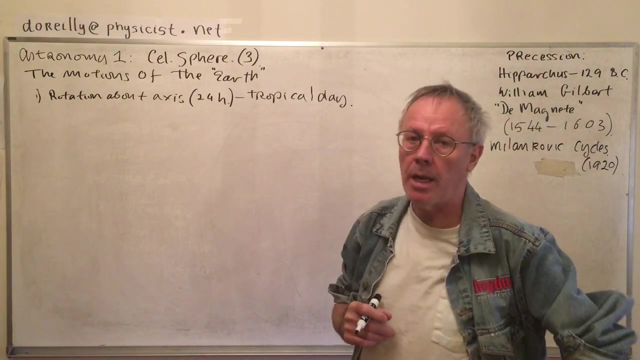 We'll talk about that in a minute. Now, the first one, of course, is the rotation about the axis. 24 hours is what it takes, And that will allow us to define the 24-hour tropical day or the hour with 3,600 seconds in it. 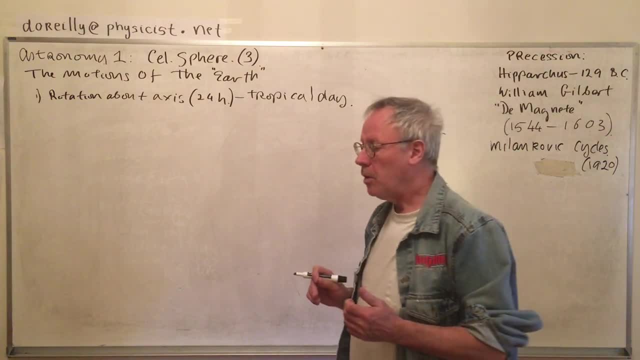 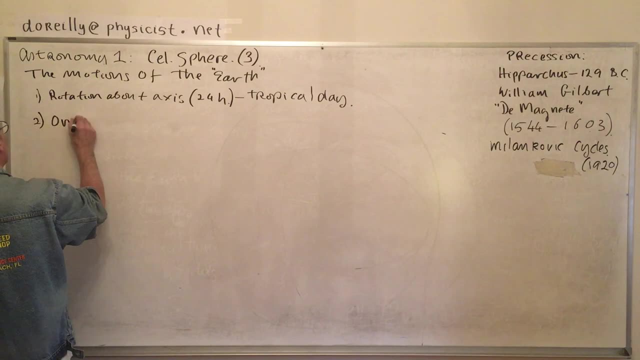 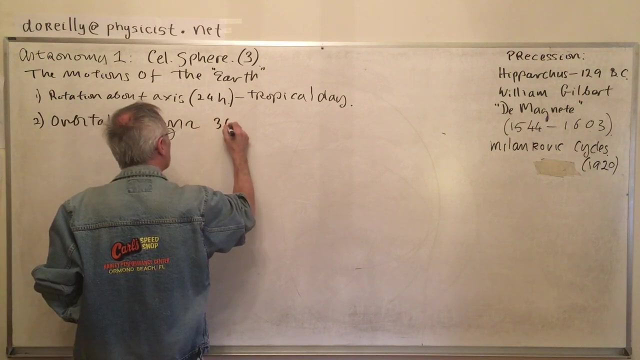 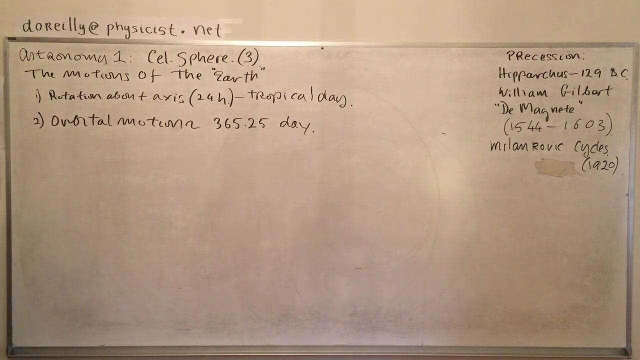 And it varies a little bit. There are variations in that, you know, depending on where the sun is in its orbit, And that way we'll be able to assassinate both about case of brain to something, And then we'll talk about moving things in the 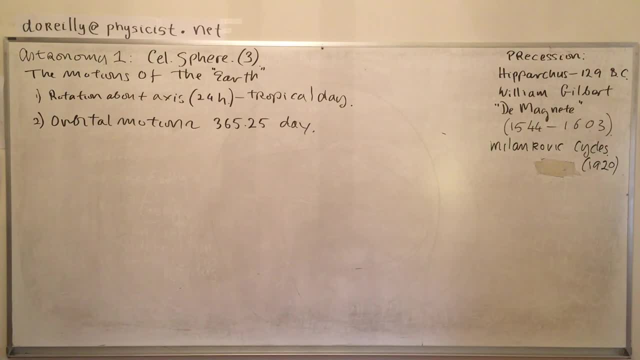 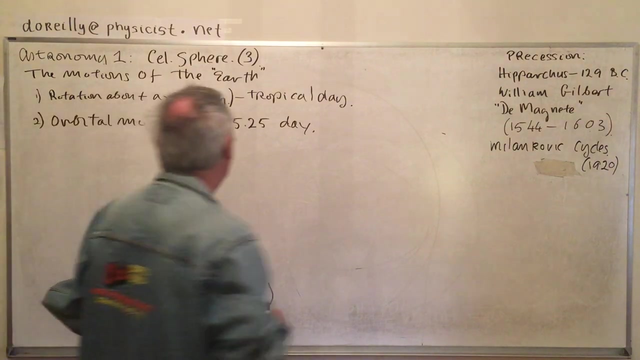 What we're looking at again is a wonderful three dimensional New York, A Guys Table. It's been exposed to the light for a long time Now, I feel, about what we'll learn about the movement of our Earth: approximately 365.25 days. I was trying to look up the exact time, or at least a 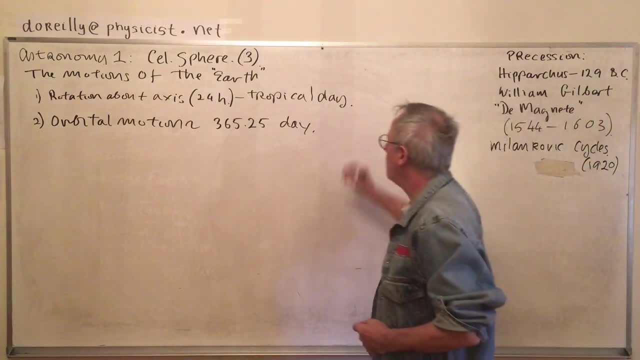 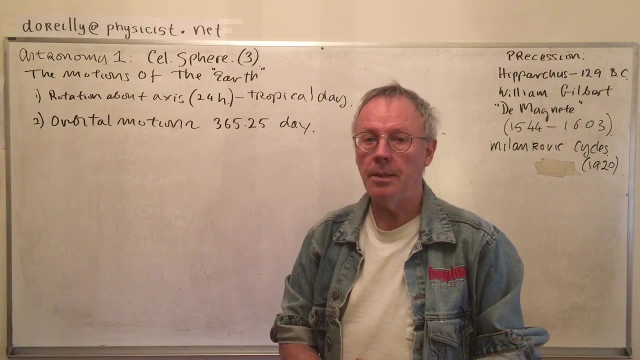 more exact figure and I just couldn't find it so quickly. So the orbital motion: the Earth goes around the Sun. Now it goes around the Sun in an ellipse, so there are variations in that motion as well. I'll come to that in a minute. 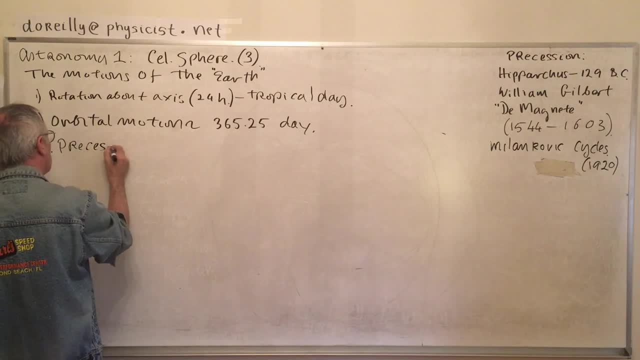 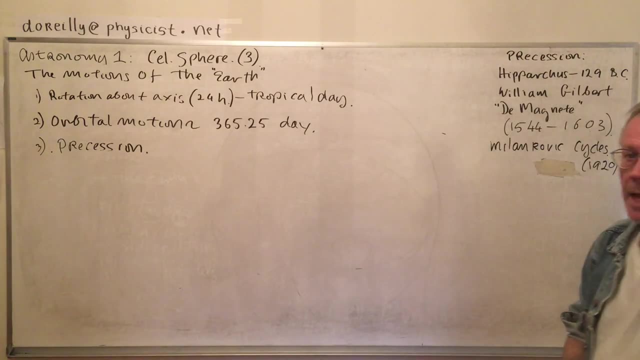 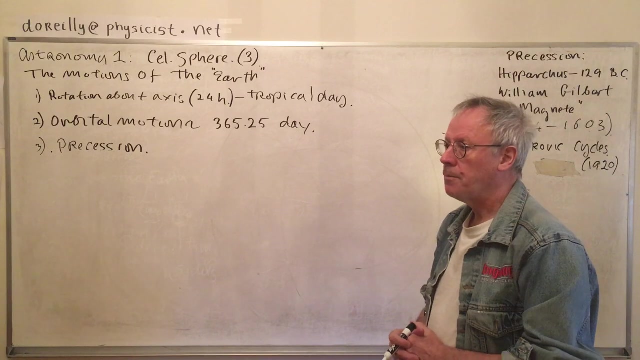 Now the next motion is Procession, actually first called precession- of the equinoxes. The equinoxes rotate around at the rate of, I think, one degree every zehn, or times in 72 years, or something like that. Alright, then, and eventually they 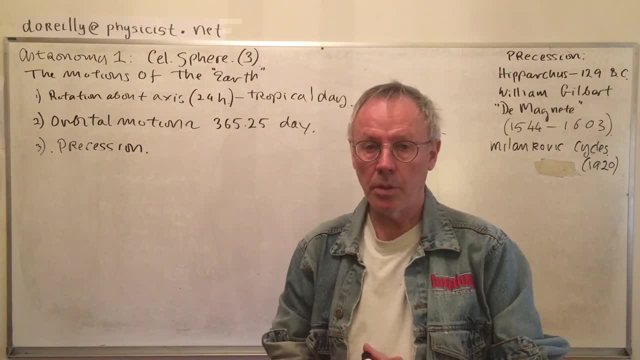 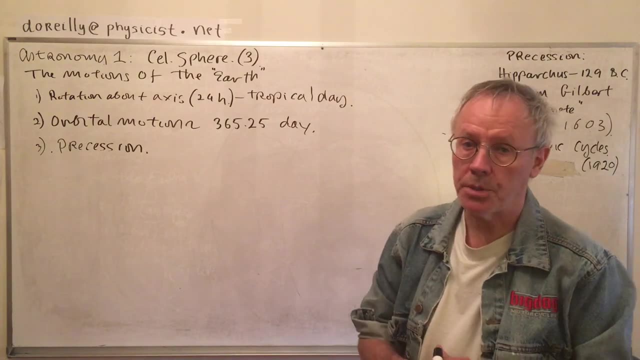 complete a cycle. Now all tops execute precessional motion. Procession of the Earth, The Earth turns The Earth. opposition, your massive force of quo. Processional motion is accompanied by another motion called nutation. That's done by TOPS. 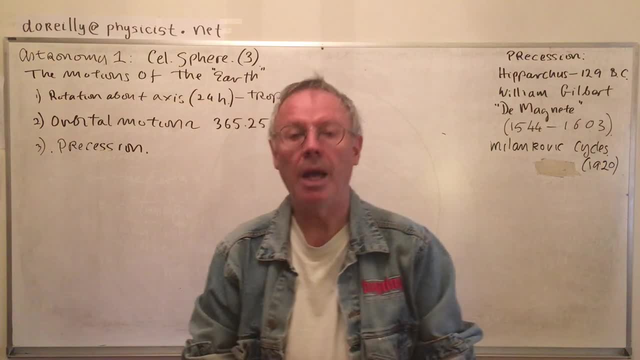 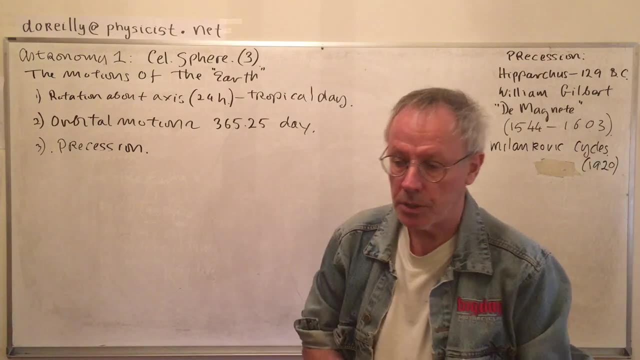 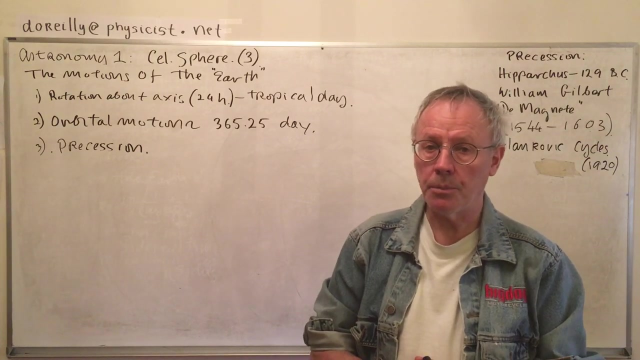 Rigid bodies And the equations of motion of rigid bodies- actually I do a class on that- are described by the Euler equations Very complicated, little equations. The Euler equations involve moments of inertia and motion of rigid bodies, But TOPS execute precession. 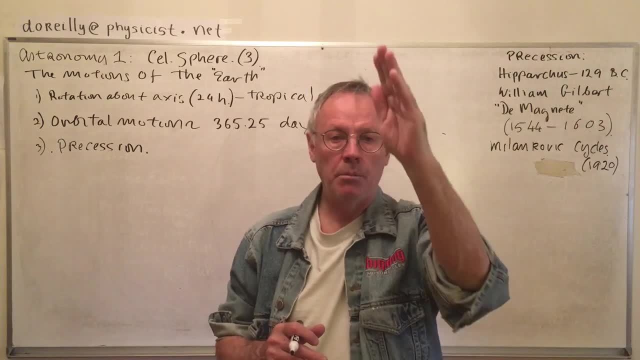 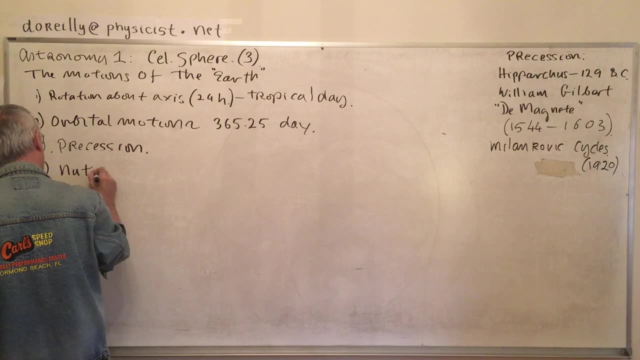 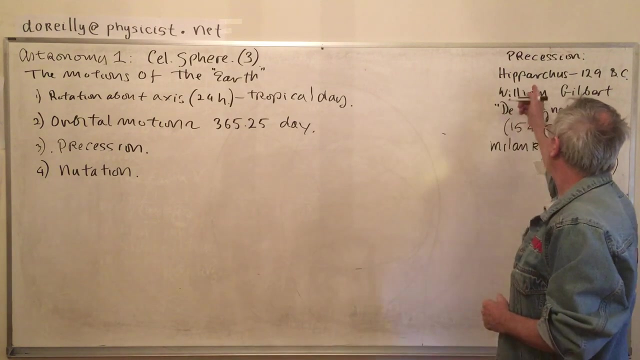 They spin on their axis and then they have a wobble. But there's another one that they do as well. I'll talk about that in a minute. The other motion associated with precession is called nutation. Now Hipparchus in around 129 BC. 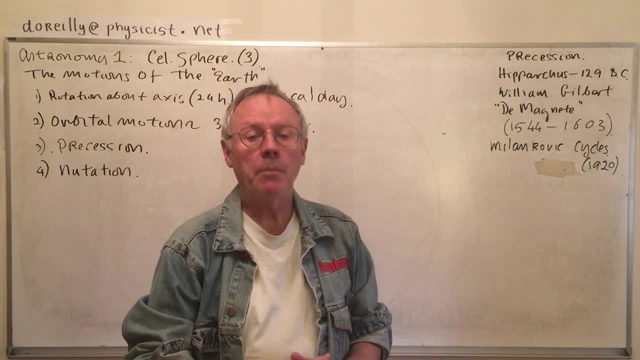 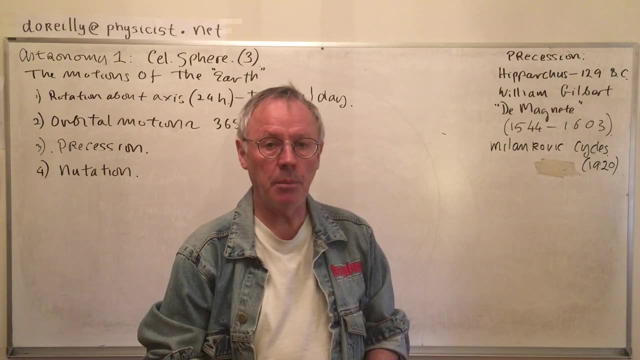 noticed first, at least that we can remember that's recorded- precession of the equinoxes. Now we didn't know why that was happening, but that was explained by William Gilbert approximately Well, at some time, let's say 1470 or something. 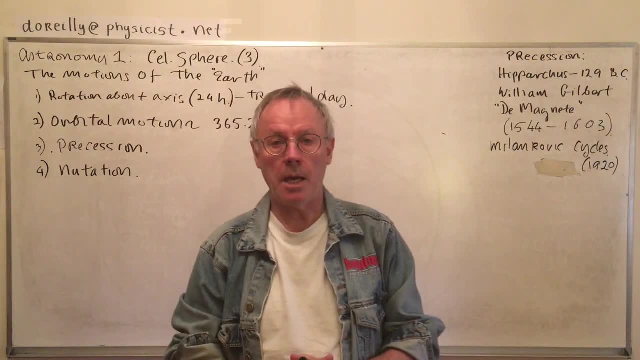 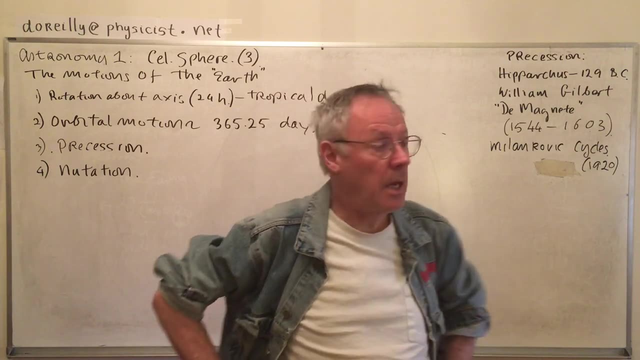 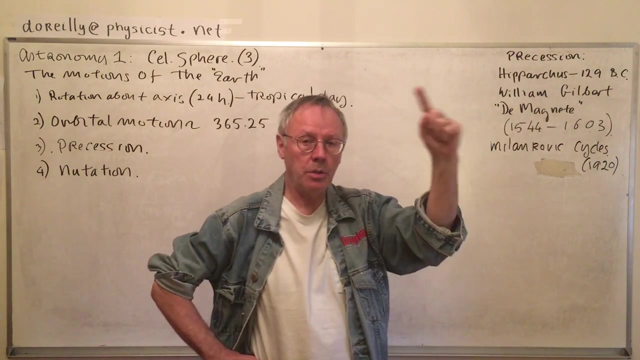 In the famous book De Magnete, The Man Before His Time- followed by Kepler very closely, by the way- Yeah, I could say a lot about that and today I won't bother. So he said that it's the same precession that exists in the topular motion. 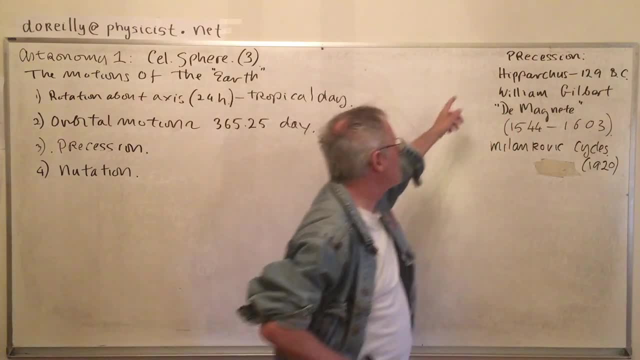 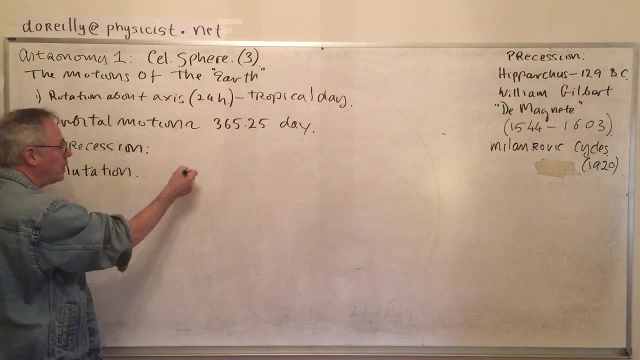 They use that word for TOPS. That causes this precession of the equinoxes. That causes this precession of the equinoxes. That causes this precession of the equinoxes, Precession of the equinoxes. So precession two things. 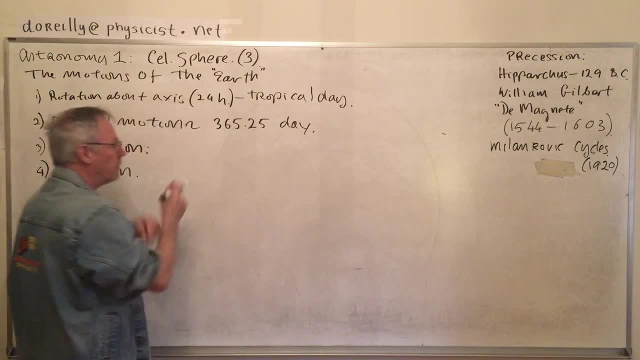 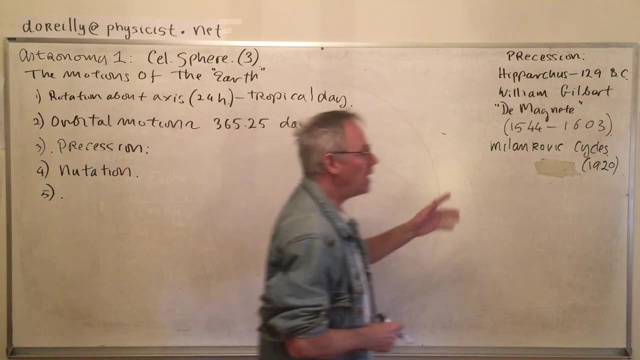 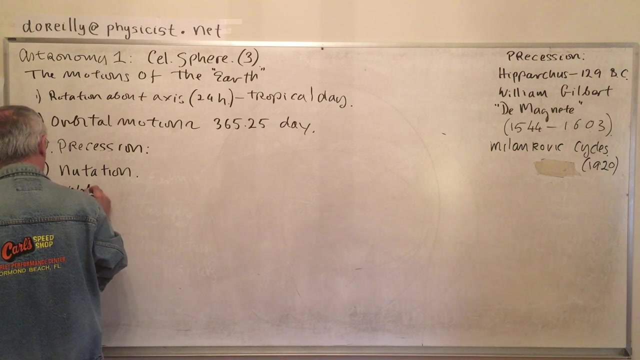 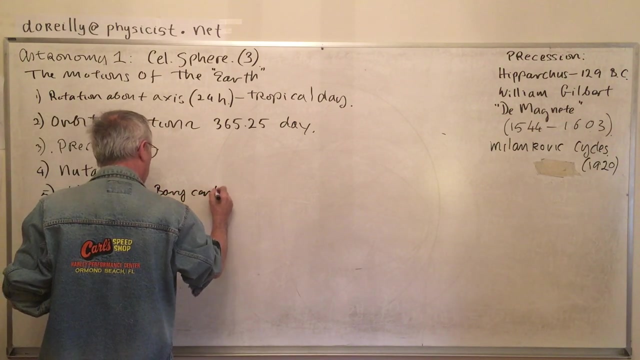 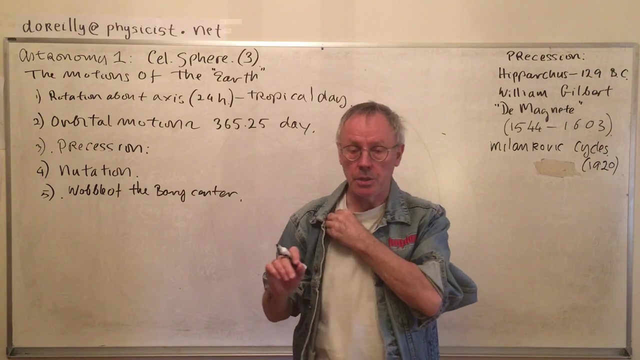 Precession of the equinoxes, precession of the top. They're both related. Nutation is a kind of a wobble. Now there's another one. The Earth and the Moon have a centre of mass about 4,000 kilometres from the Earth's axis. Something like that. 3,000, I don't know. But the Earth doesn't go around on its own axis. It goes around with this little bit of a wobble. As it keeps going around in its orbit, this wobble shows up as an extra motion. 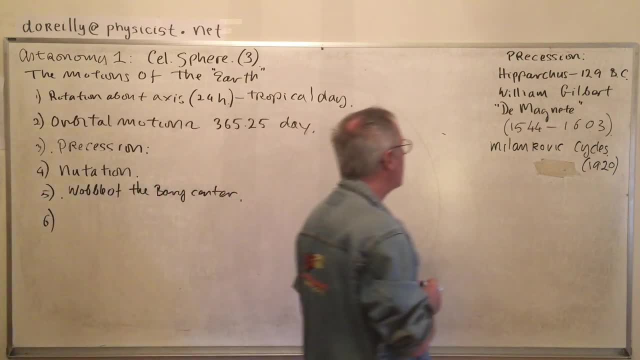 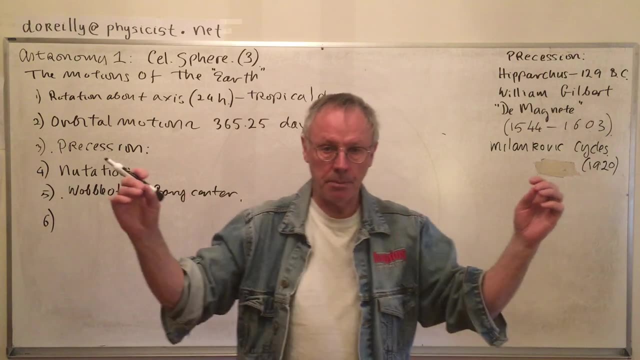 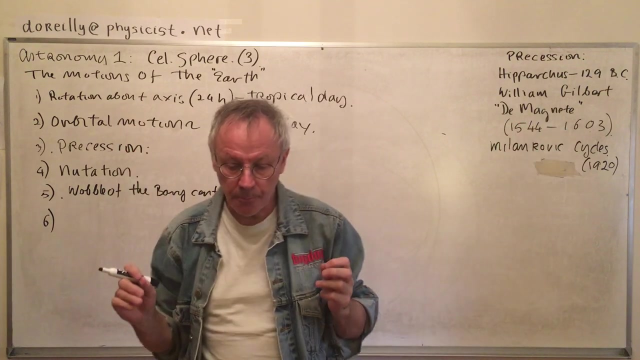 Now another motion. let's see what I can put in The Milankovitch cycles. Now the Earth's orbit is elliptical. Well, wait a minute. at present it varies between 94.5 million miles and 91.5 million miles approximately. 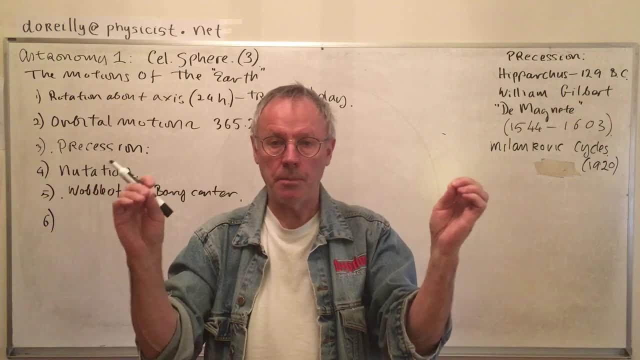 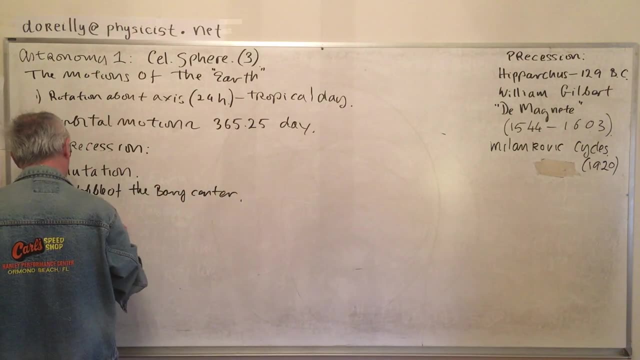 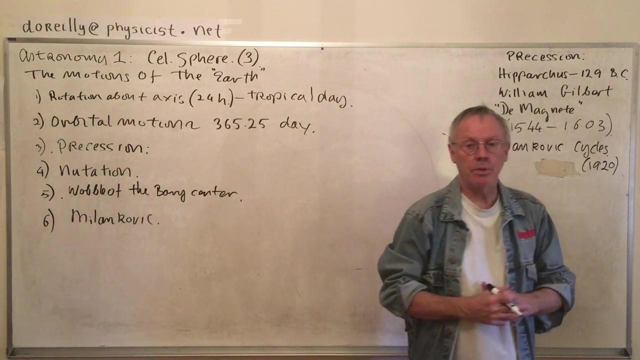 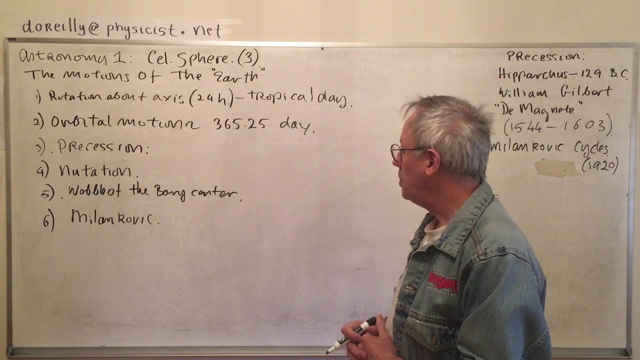 At some point it becomes almost circular. This has an effect on the Earth And on the seasons. Milankovitch motion: This was discussed only as recently as the 1920s. So there are six motions: Rotation of the axis, orbital motion, precession, mutation, wobble of the barycentre. Milankovitch. 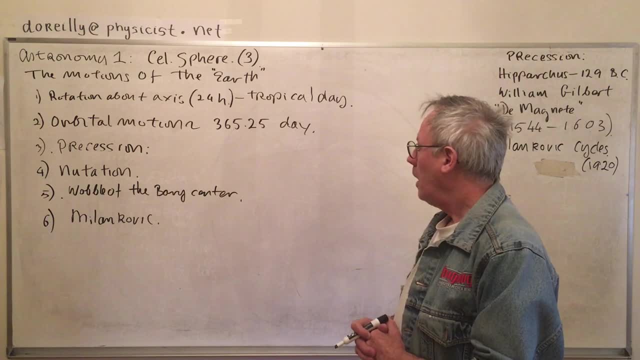 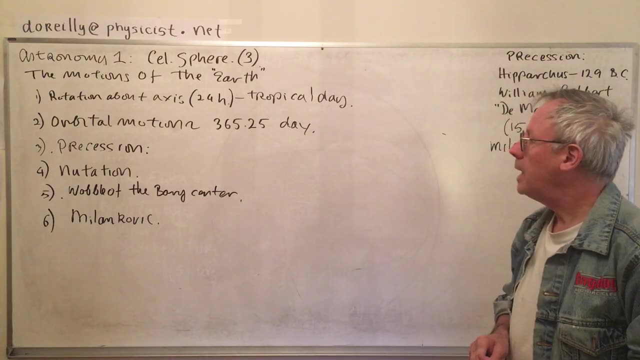 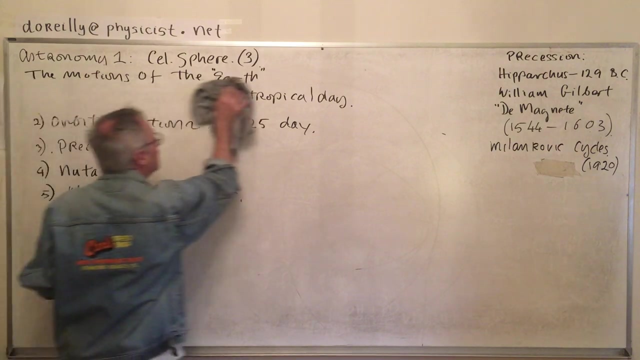 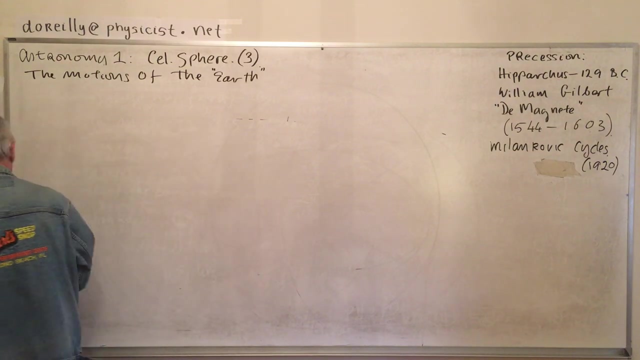 What else could I put in there? I had seven the last time, But that'll do us for now. So let's look a little bit more closely at these motions. Rotation of the axis: That's a pretty easy one, But there's a complication. 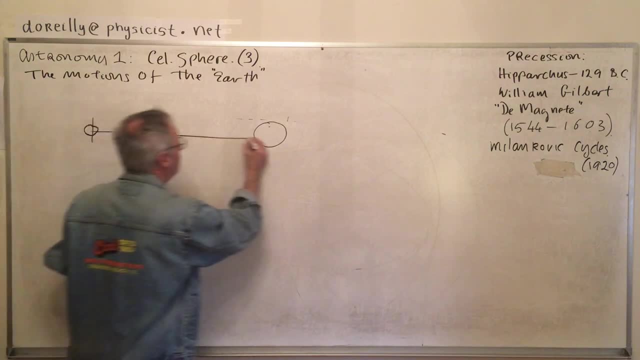 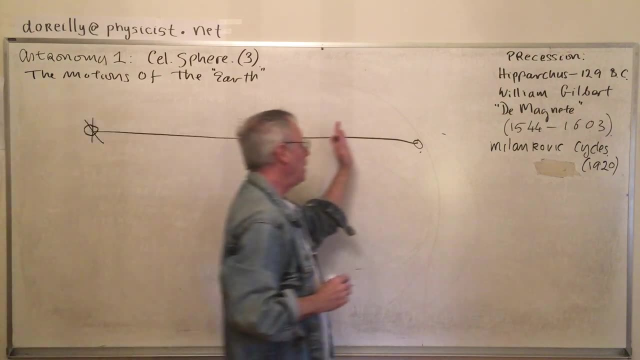 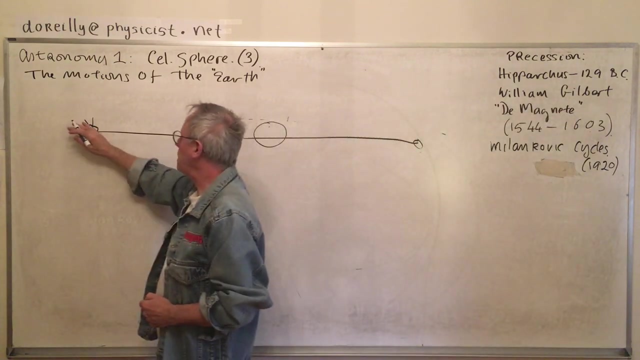 The complication is that in the orbital plane the Earth's axis is not vertical, it's tilted, So that results in the Earth with the Northern Hemisphere facing the Sun in summer and facing away from the Sun in the Northern Hemisphere in winter, and vice versa for downstairs. 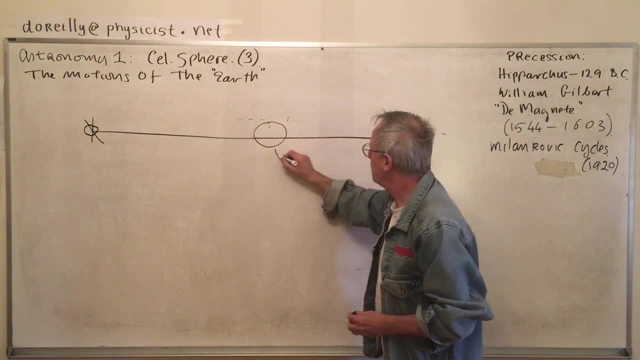 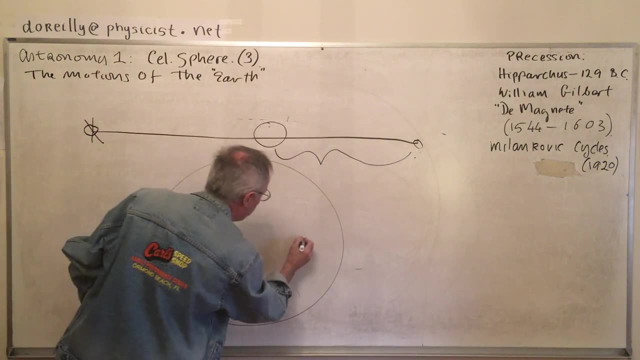 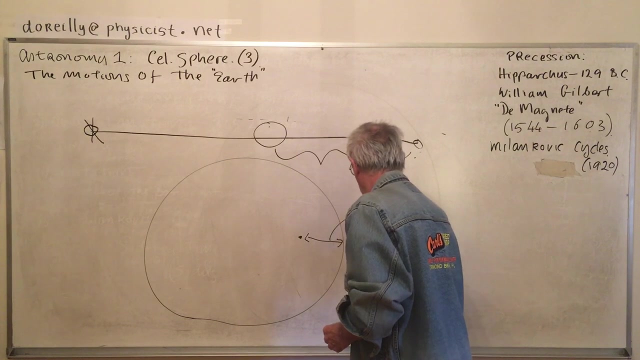 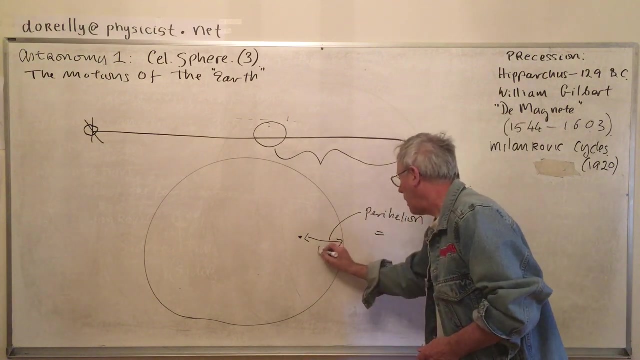 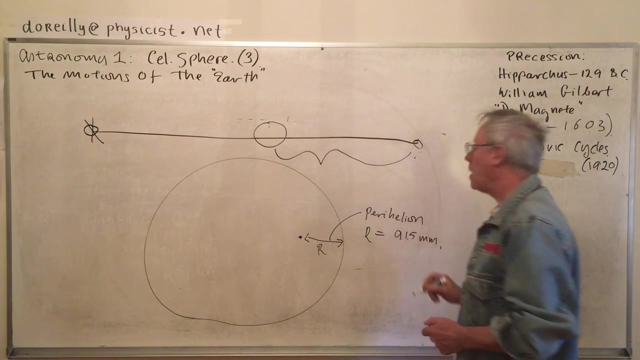 The rods also affect you to this distance, because the orbit is in ellipse. This is a little bit more complicated. This is an exaggeration. So at perihelion, at perihelion, the orbital radius is approximately 91.5 million miles. 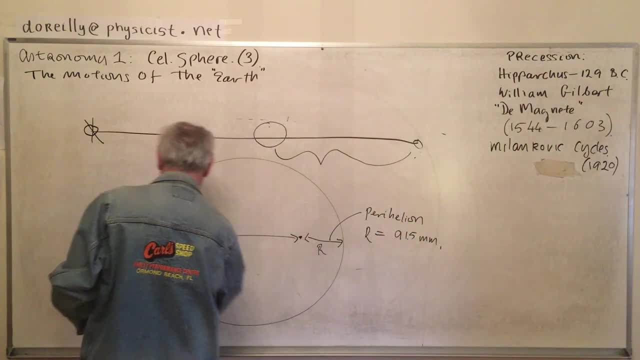 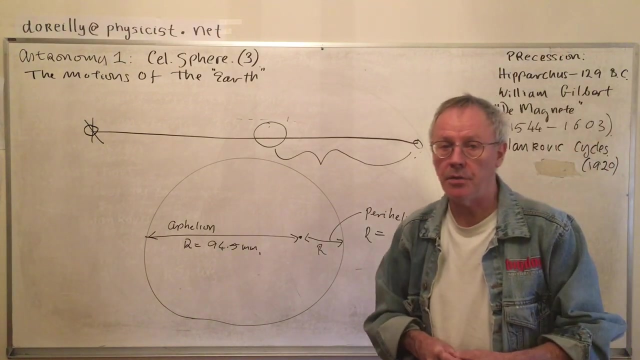 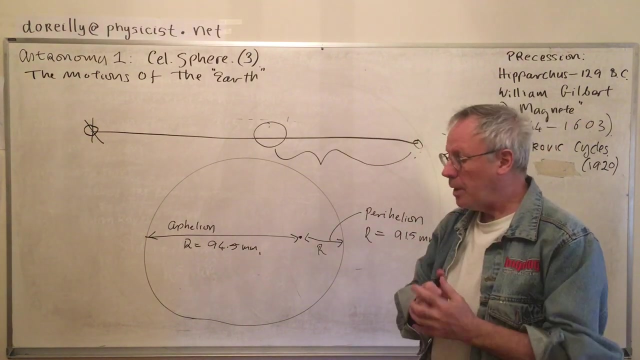 And at aphelion it's 94.5 million miles, And we generally say that the average orbital distance to the Sun is 93 million miles. But this distance, the difference of 3 million miles, makes a difference to the amount of heat. 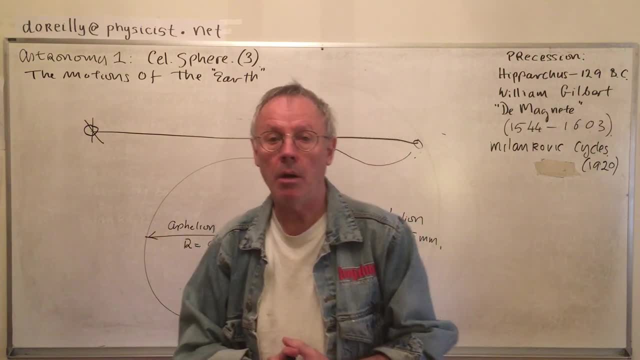 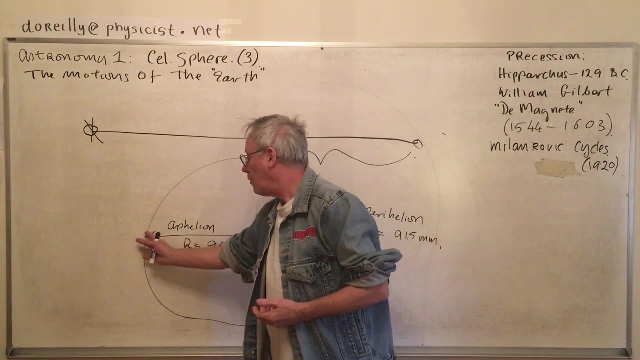 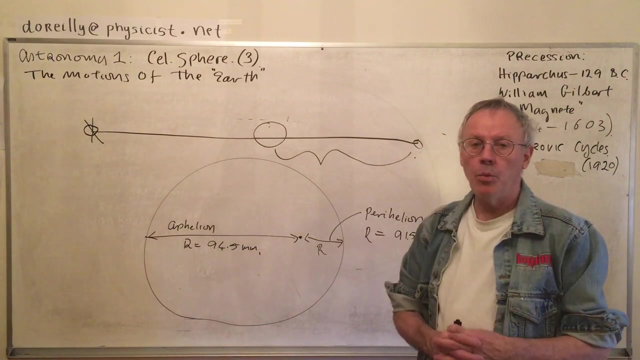 that the Earth will absorb from the Sun. Due to the inverse square law, it's sizeable right. That means that if you have a summer in the Northern Hemisphere- over here, compared to over here right- there's going to be a weather difference. 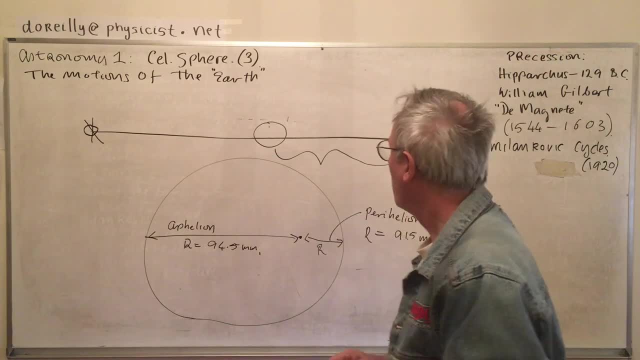 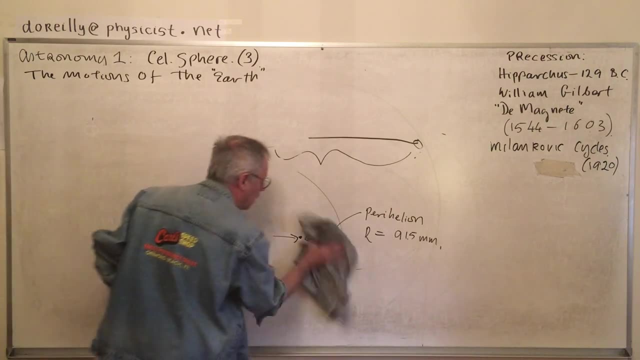 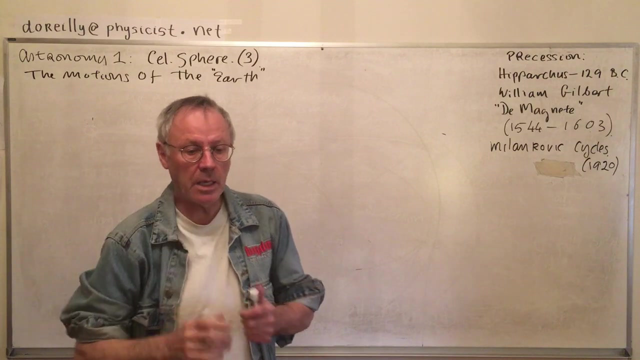 And that's food for thought for a whole class. So that's the orbital motion. Let's look at precession now. Now there are the two main motions. If I want to work out time, a thing called sidereal time, I can approximate it just by considering it. 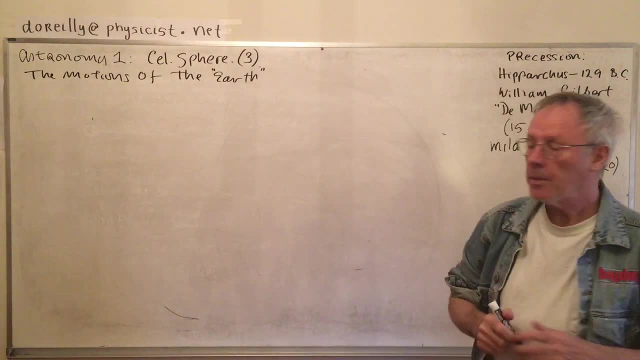 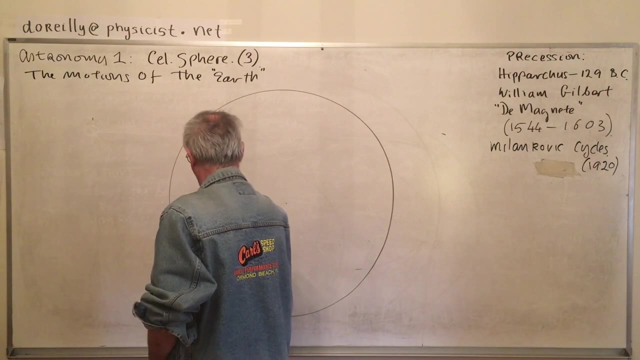 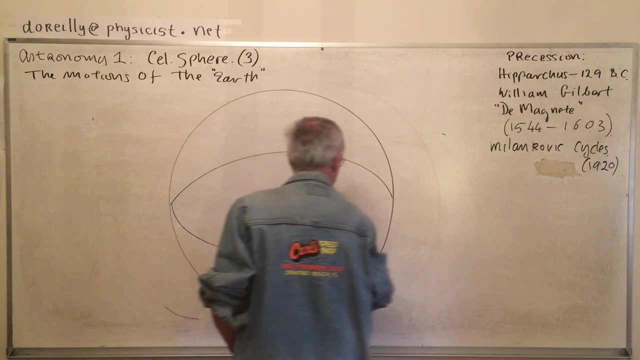 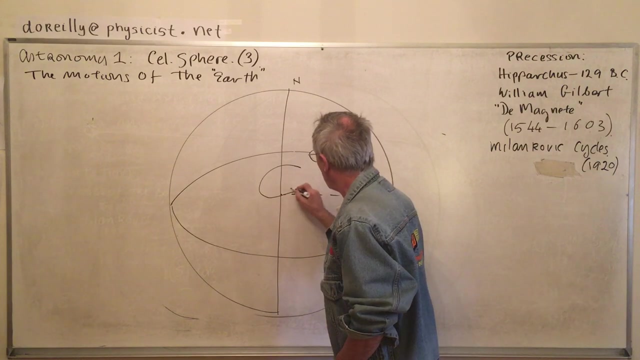 Because the next motions are small. Now, the first one I'm going to look at is precession. Now, let's put the Earth's axis in like that, And the Earth is going to be moving anticlockwise if you look down on it. 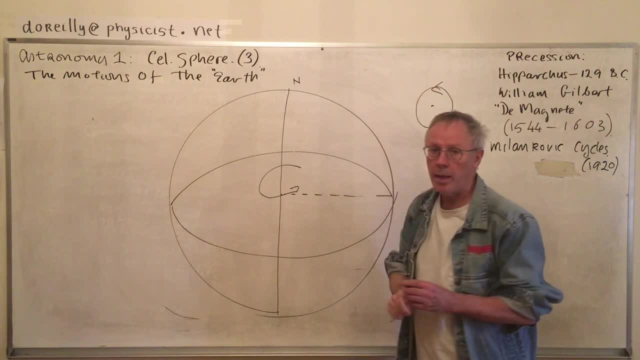 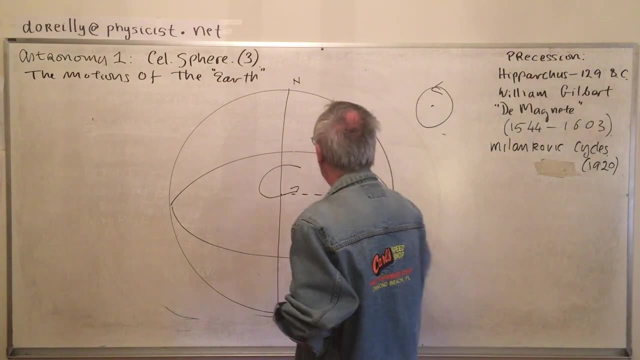 If you look down on the Earth at the North Pole, there the Earth is turning anticlockwise. That ensures that the Sun, as we know it, rises in the East and sets in the West. Okay, so what's precession? 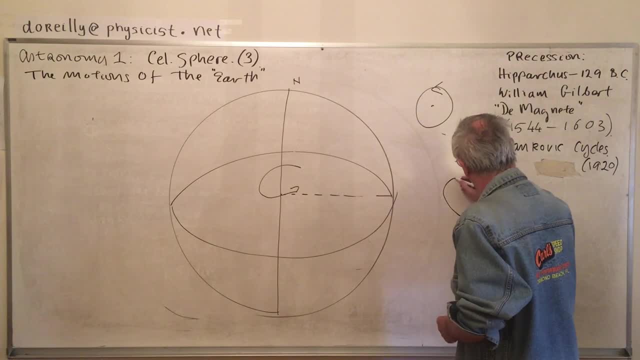 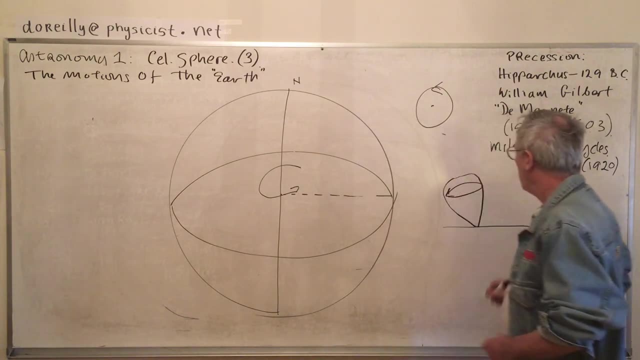 Well, all tops here's a top, And if you spin a top and it starts rotating, we have the first motion of the top as being the rotation. So the Earth is a top right, It's tilted on its axis. 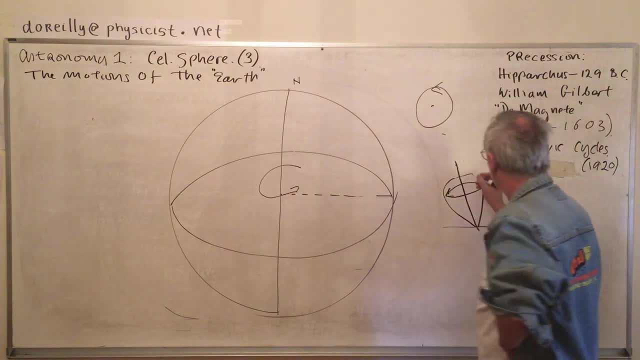 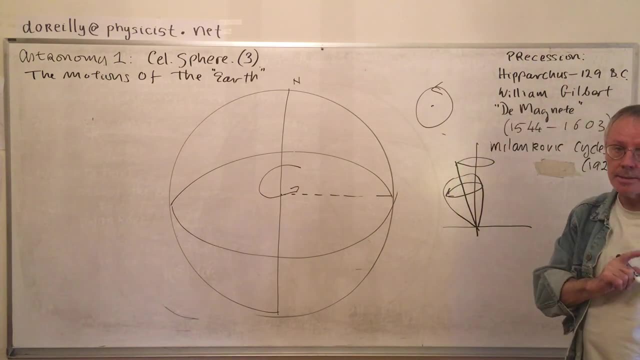 But that's a separate idea. This is the axis. The axis of rotation on the top rotates about its own axis, This one. So if you're rotating a top, this rotation is called precession, The Earth's axis. so we have Polaris at the top of it at the moment. 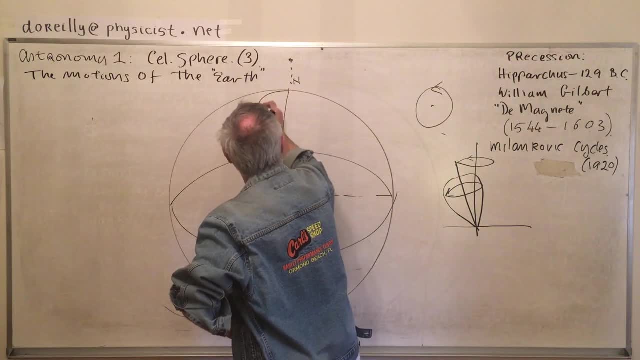 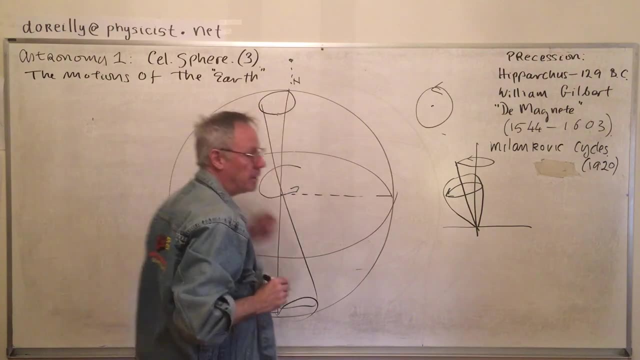 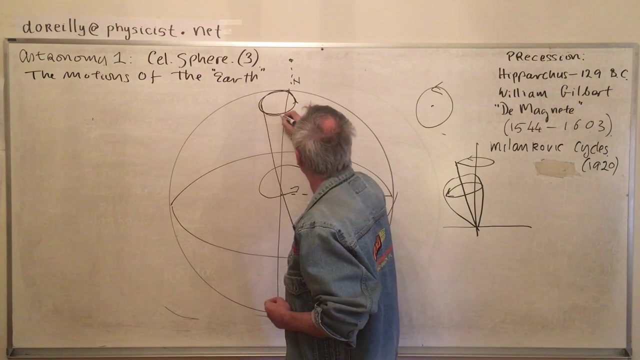 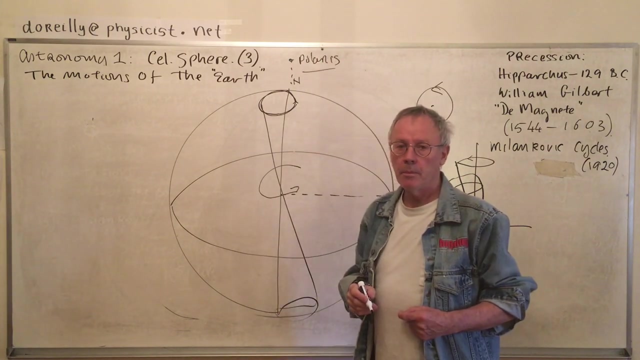 it also has a precession And that precession generates a cone, This cone, this tip of the cone, the cycle that the axis goes through. so if we are at Polaris right now, Polaris being a North Star 12,000 years from now, 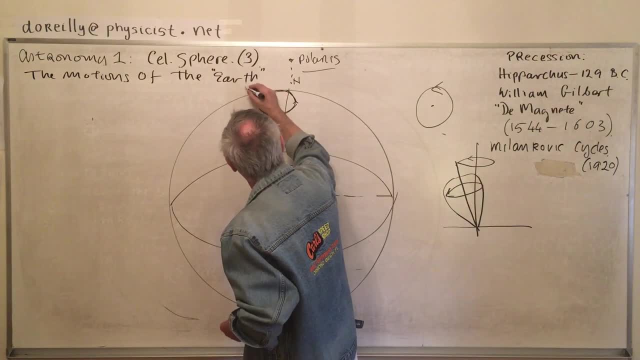 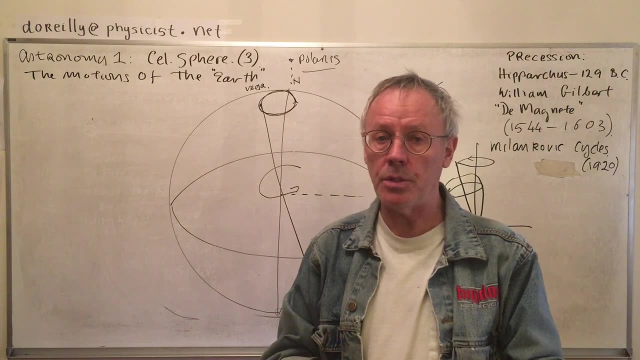 it will be Vega. The pole of the Earth will be pointed towards Vega, A different star, And in between- who knows, It's approximately 26 or 27,000 years- I forget- For this cycle to take place 26,000, let's say years. 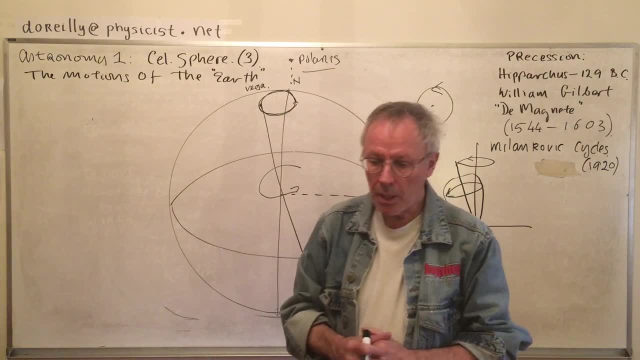 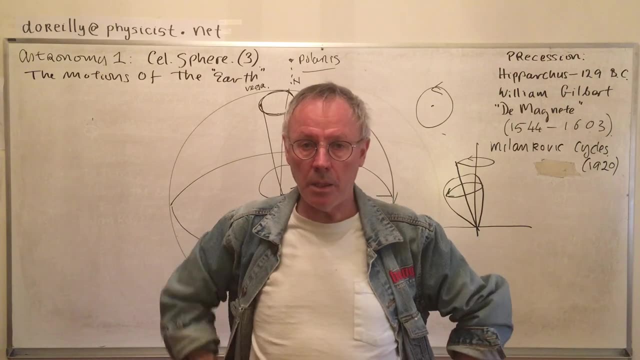 Now, that makes a big difference to weather on the Earth, but it also makes other difference. Here's an example. Okay, There is an observatory in Ireland called Newgrange and it has a passage way down deep and the observatory, by the way, 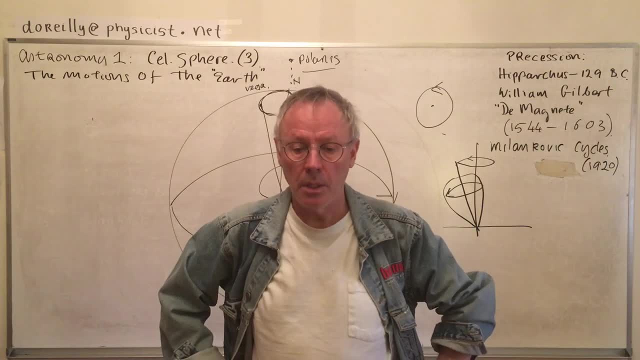 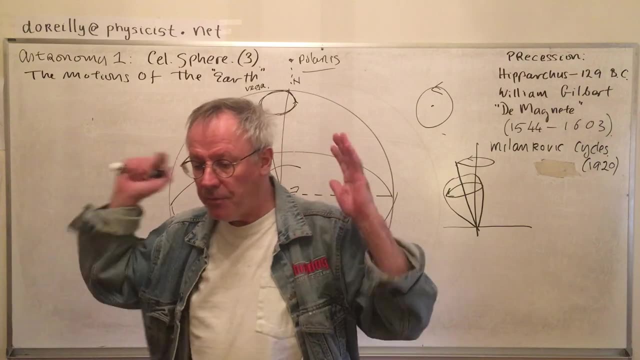 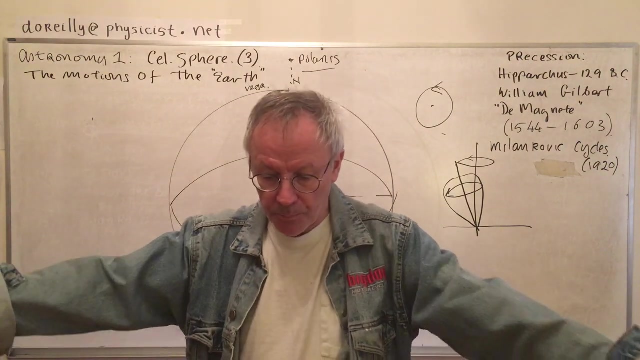 looks like it was made yesterday. It's an underground observatory. Archaeologists can be crazy. sometimes Everything for them is a tomb. and this was supposedly a tomb. It's not a tomb. And then down at the bottom of the tunnel. 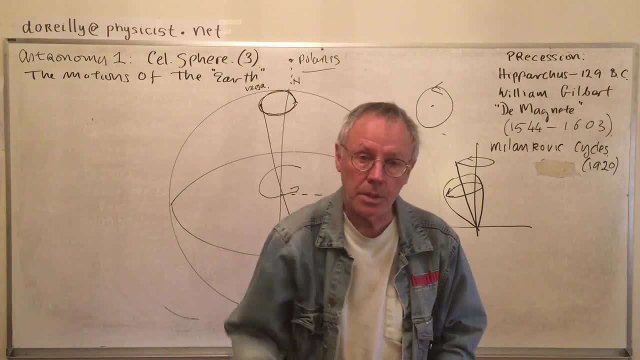 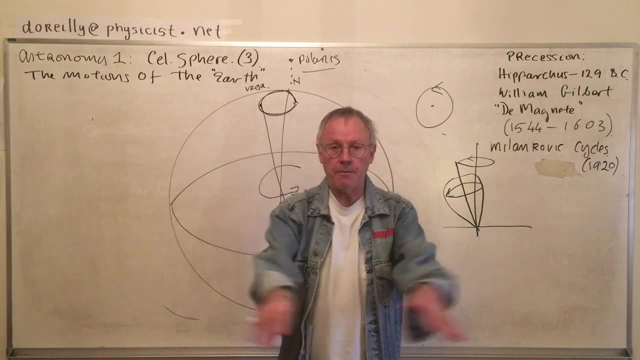 on the solstice. the Earth can get the Sun, can get its sunlight all the way down into the main chamber. In the main chamber is a huge stone bowl, concave. Now I don't, I haven't heard it said. 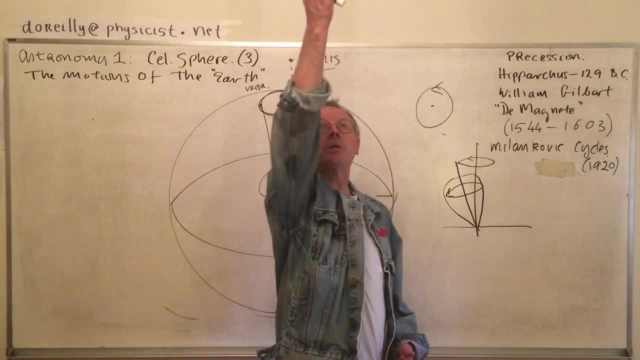 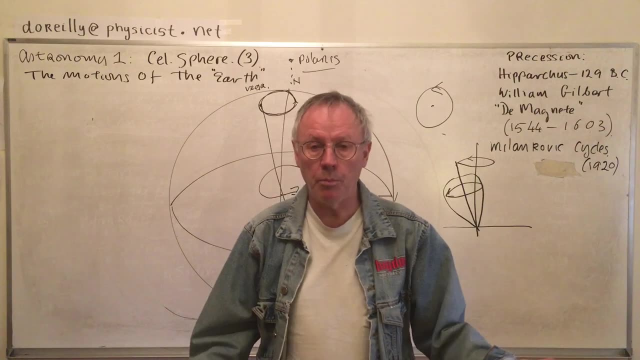 but oh yeah, when the Sun comes in on the solstice it lights up the ceiling, but it would do it even more so if they put water in there. That Sun would be reflected onto the ceiling and it does it very closely. 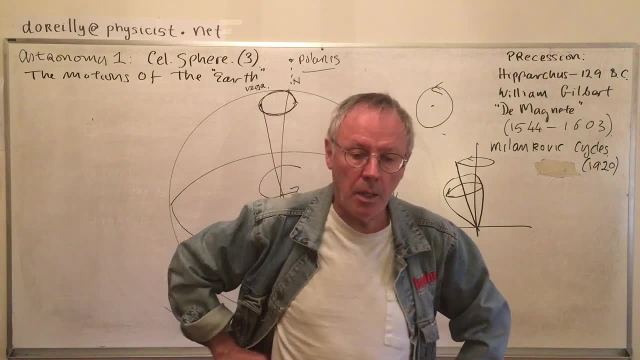 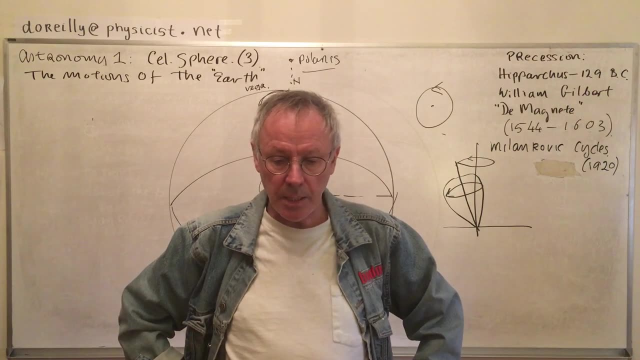 but it misses it by about seven minutes. You know, this event happens seven or eight minutes past midday on the summer solstice. That is the lighting of the tomb and people say, well, that was a pretty good building anyway for 5,000 years ago. 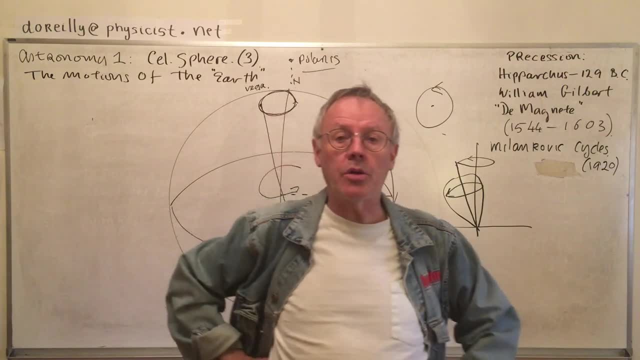 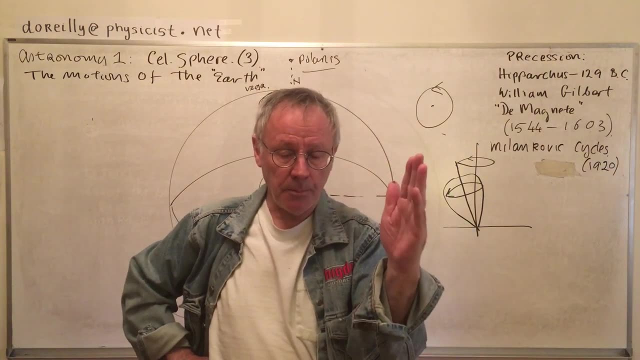 But wait a minute. 5,000 years ago, That's a quarter of a procession. If you take that into account, then the Earth's axis will have tilted a little bit and the light will shine exactly, or at least more closely. 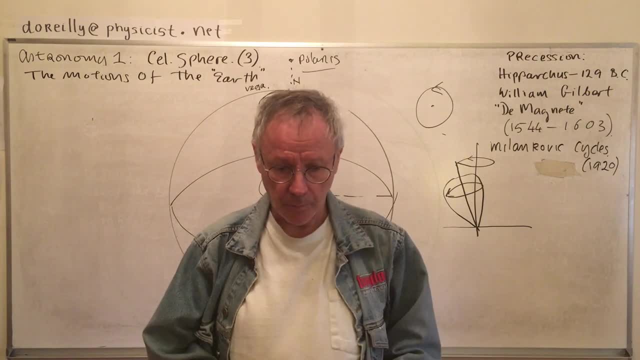 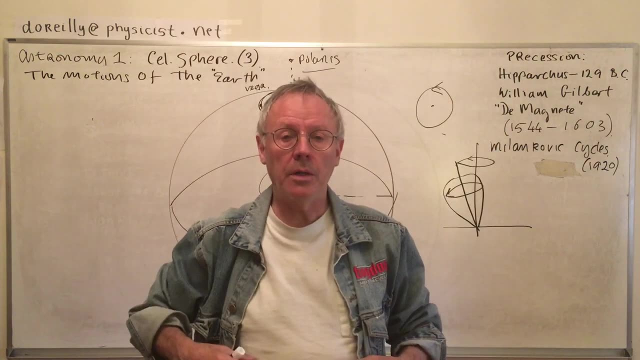 on this magic bowl, And at midday, closer to midday, 5,000 years ago, when the observatory was first built, the light would hit the room, the roof, much more closely. All right, So that's the effect of procession. 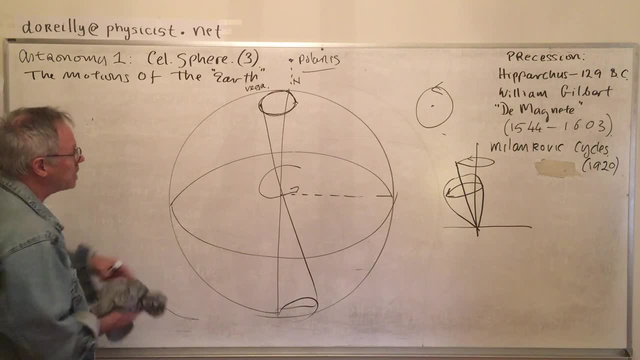 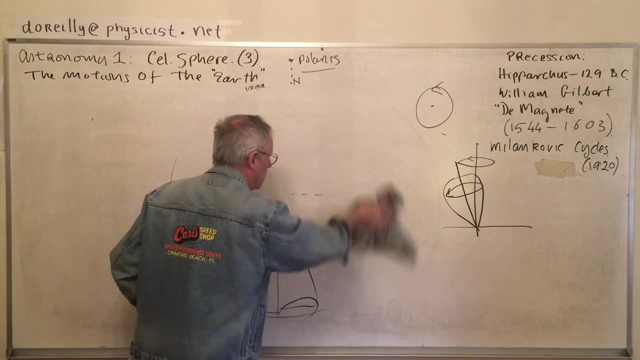 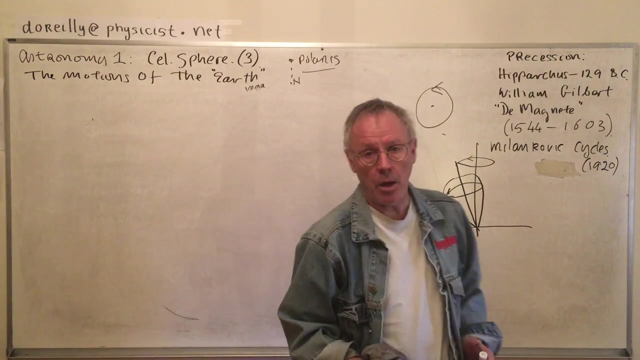 Now, procession of the axis here results in procession of the equinoxes. That means day and night are of equal length at one particular day, Let's say the 21st of March right now, But you know, in 1,500 years' time. 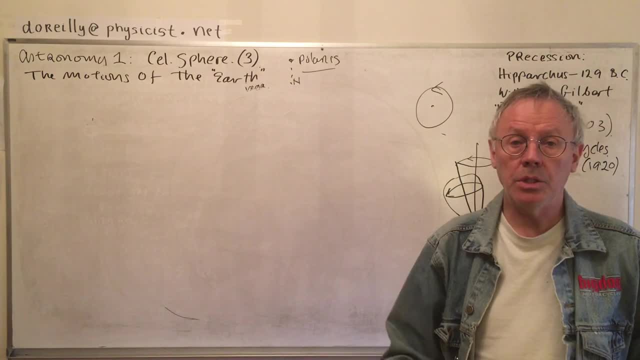 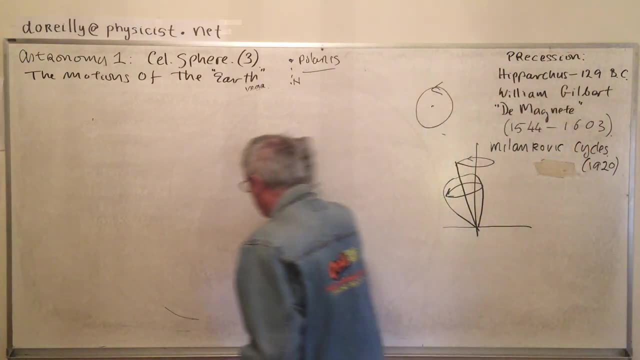 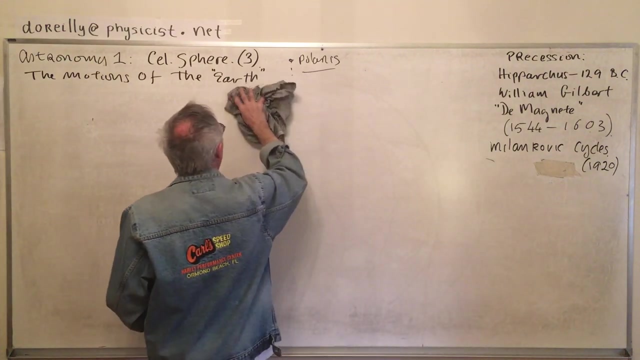 it could be the 22nd of March, 1,000 years, 1,000 years, 23rd of March, and so on, over that 26,000-year cycle procession of the equinoxes, Now nutation. 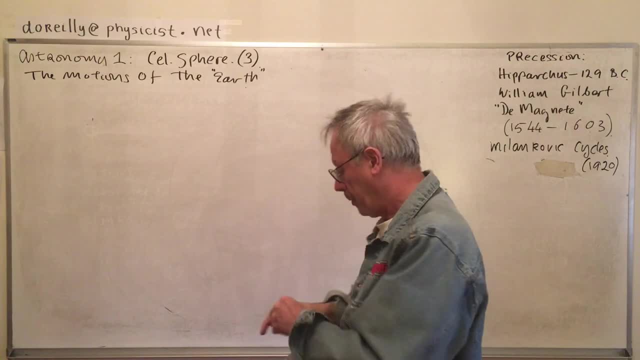 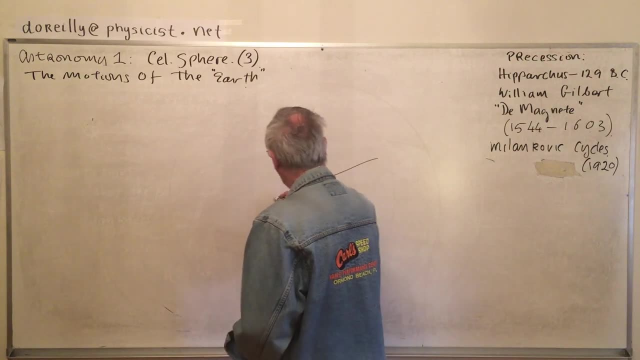 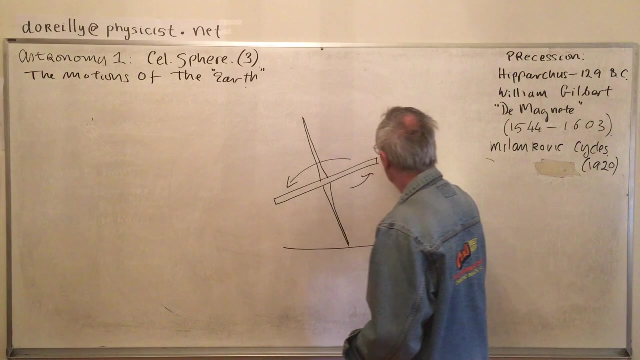 Nutation is yet another complication of emotion. Okay, let's make a top that looks like this And let's give it an axis, So a top rotates. that way, We put all the mass in here, So it's spinning. The axis of the top rotates. 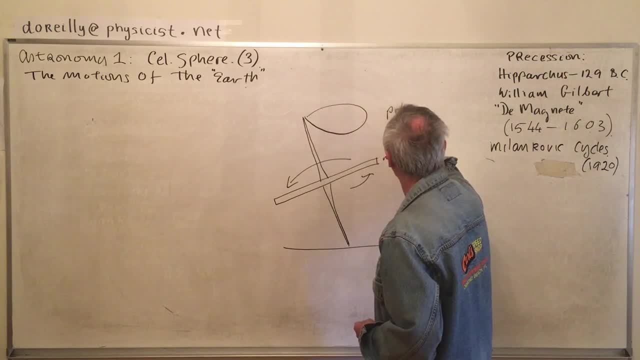 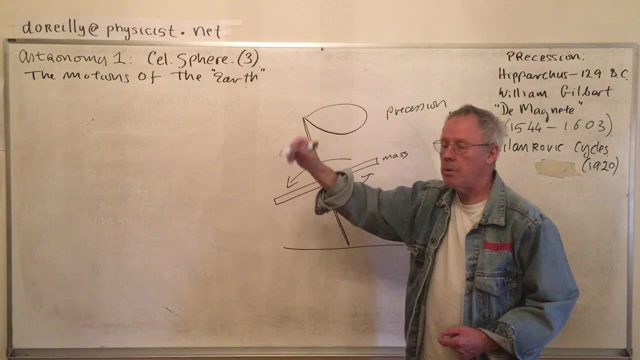 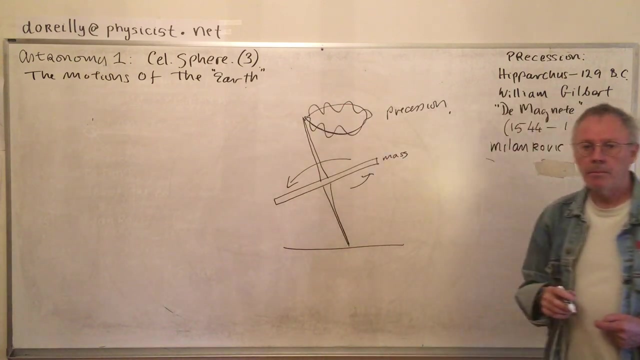 according to the procession that I told you, But there's another one. As it's processing, it also wobbles. The tip of it goes up and down. I'm sure you've seen that. yeah, Now it could come up and down. 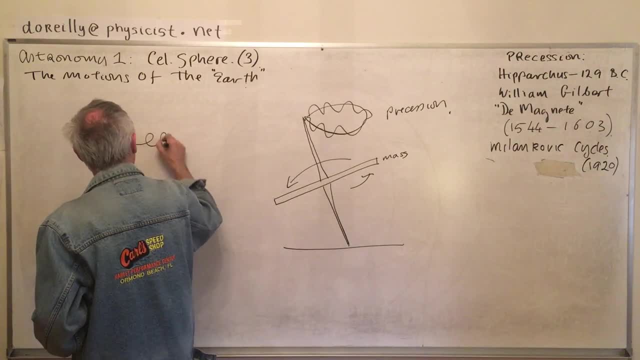 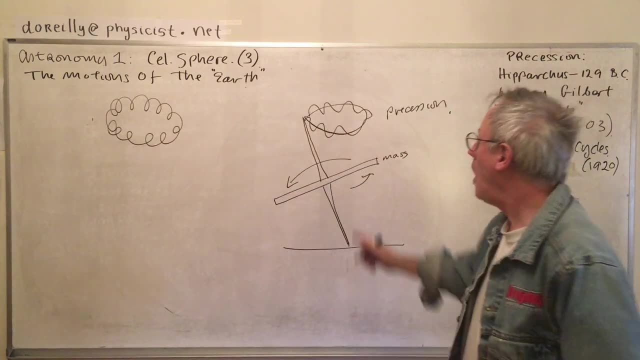 in the sinusoidal cycle, or it could do something like this. Well, the Earth is no different. It has its own wobble of this rotation. The Earth is doing this all the way around in a cycle for 27,000 years. 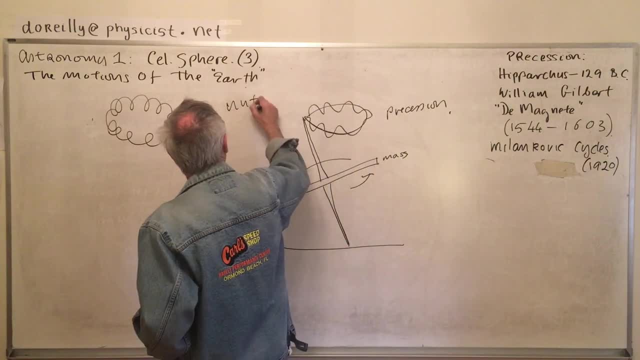 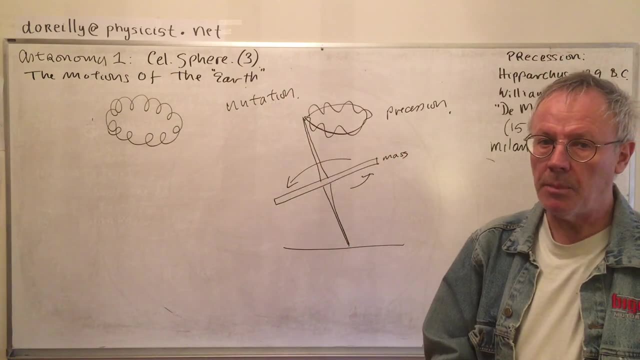 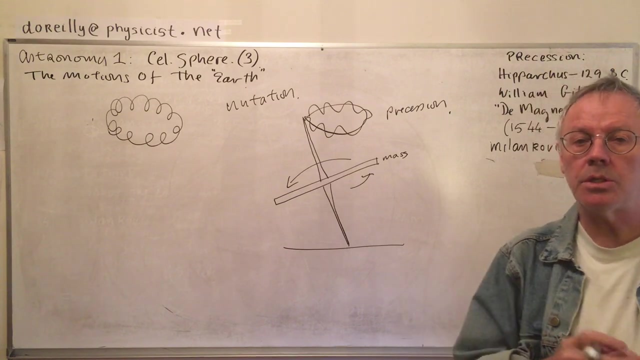 and that's called nutation. All tops do it. Oh, it's going to get more complicated than that. Remember I said that the Earth's Earth is not just the Earth, It's an Earth-Moon system, So that nutation is not so simple to figure out. 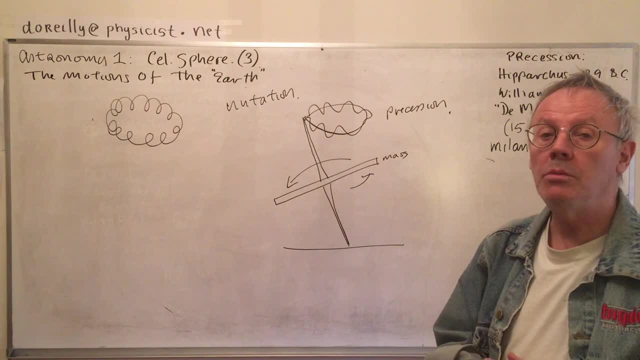 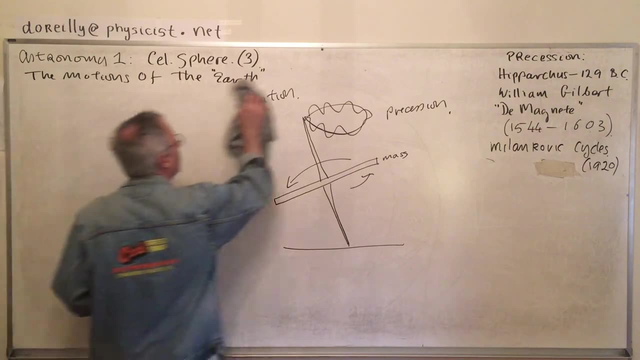 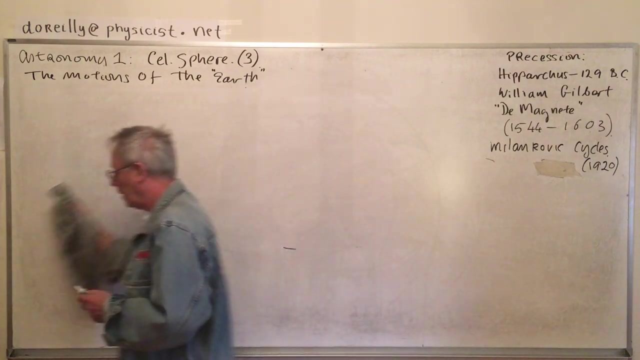 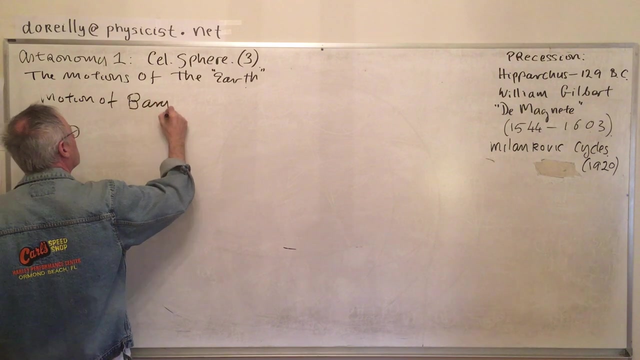 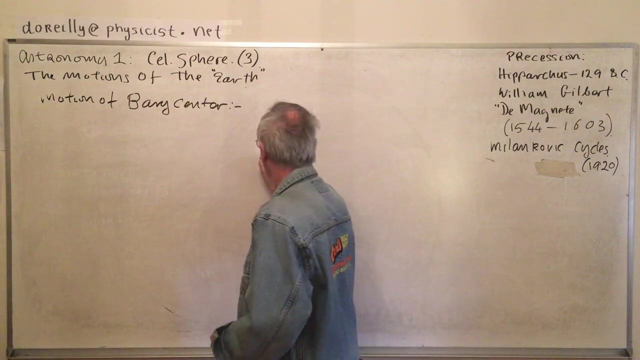 due to the complications introduced by the Moon, being dragged along with us. So the next thing we look at is the wobble of the barycenter. Oh, what's that, The barycenter? Okay, We'll take a sphere and we'll join it to another sphere. 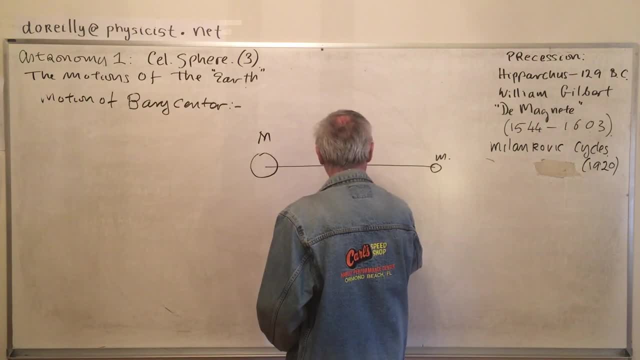 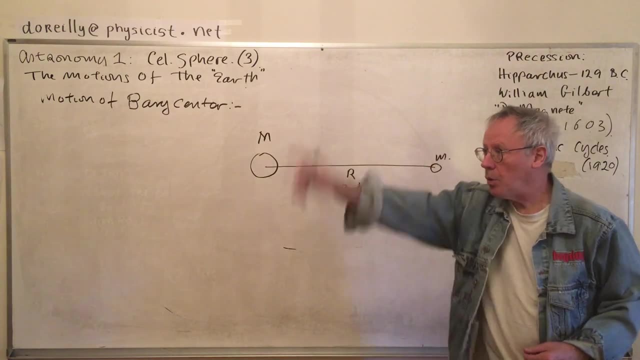 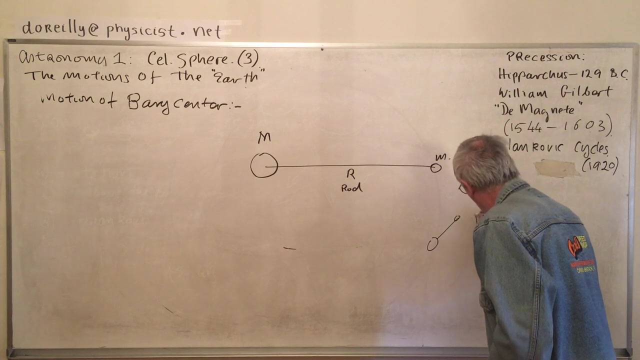 and they have masses m and m and a rod Which is massless connects them. Now we put them into a rotation, We throw them. So we throw them across the room, But really what we track is when you go across the room. 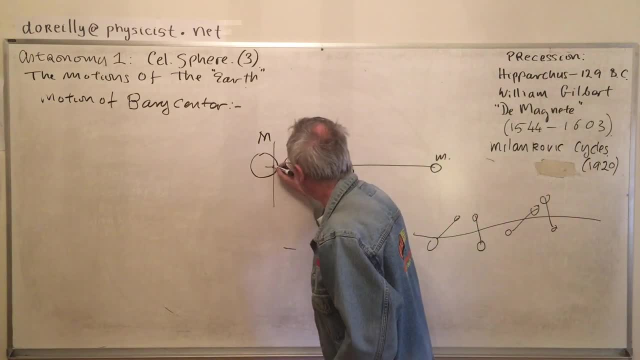 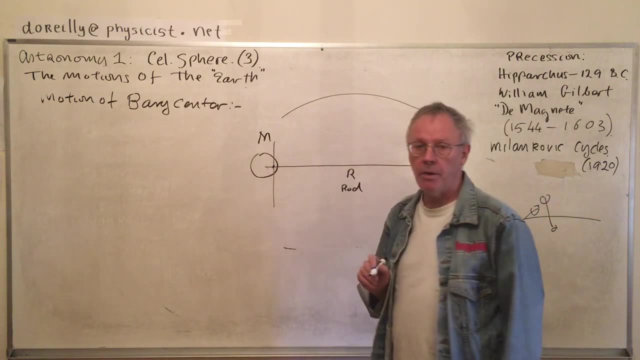 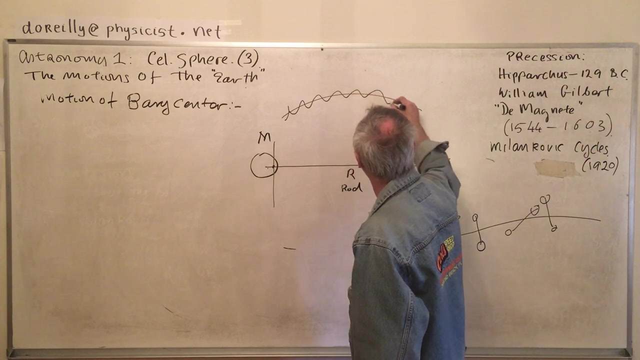 is the motion of the center of mass. The center of mass generates a parabolic path, But the individual masses do not generate a parabolic path because they're twisting. This one would generate a path that goes like this, And so would this one. 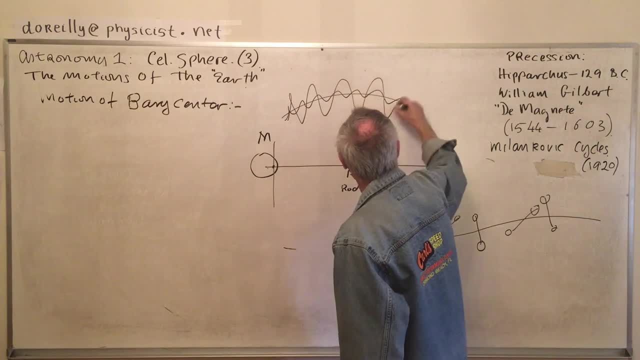 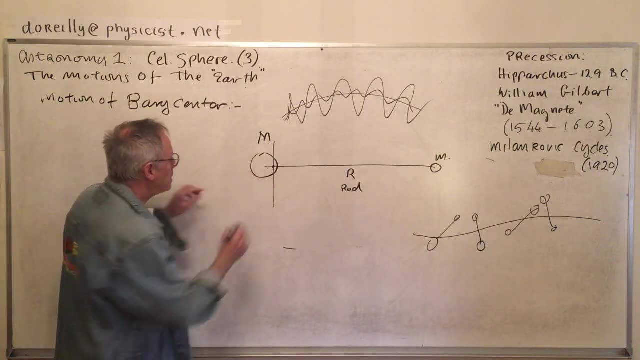 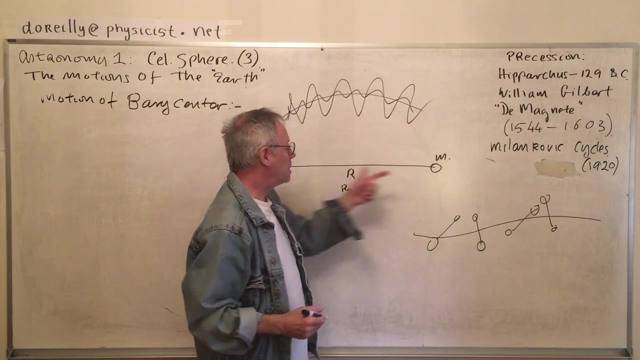 but with a bigger amplitude. So this is the path of these two guys separately. This is the barycenter. The barycenter moves on a smooth curve, but the objects don't. They're doing a wobble. What does the Earth do? 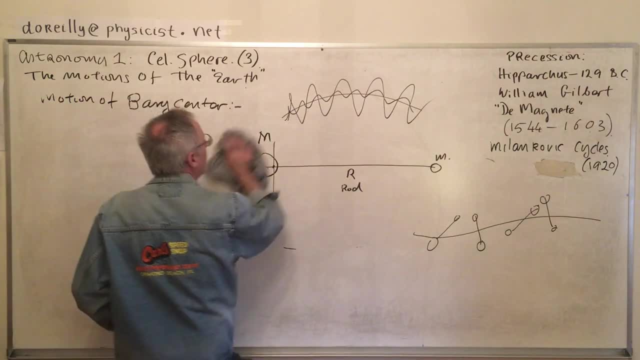 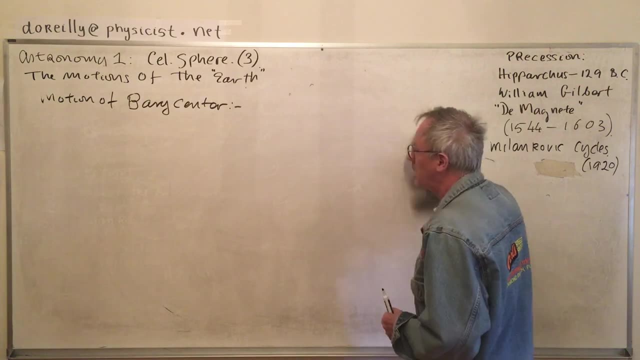 Same thing. Now, I don't know, I think it's. is it 22 days or something that this cycle happens? the time it takes for the Earth and the Sun to mutually orbit each other. Is it 22 days? I can't remember. 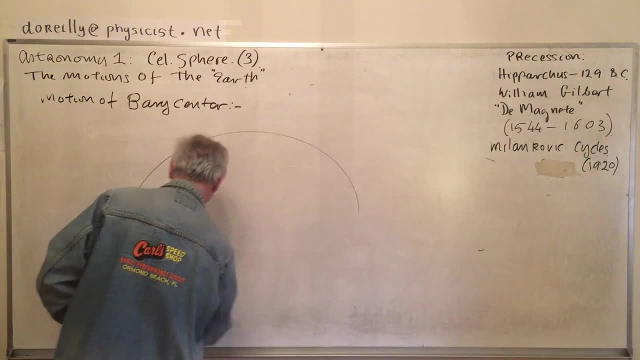 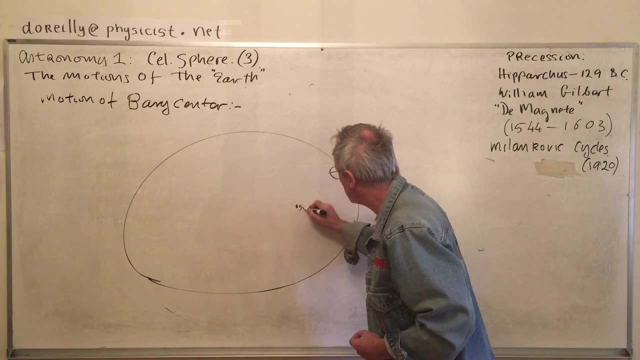 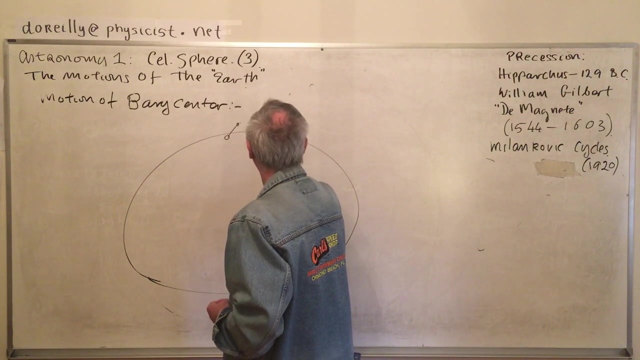 So let's suppose we have the Earth's orbit- The Earth's orbit isn't in this case an exaggerated ellipse- with the Sun at the center, And here is the Earth-Moon system, once again exaggerated, And so on and so forth. 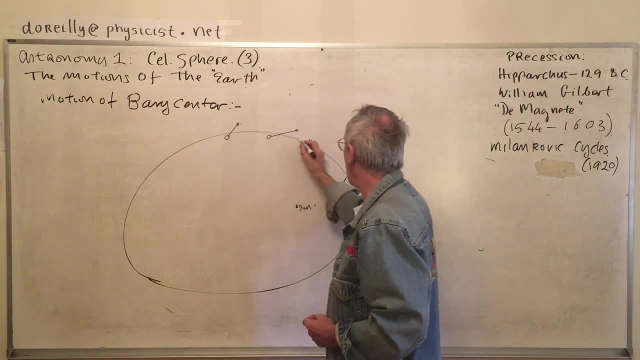 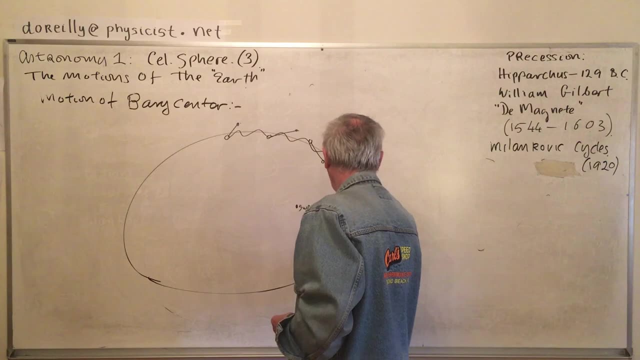 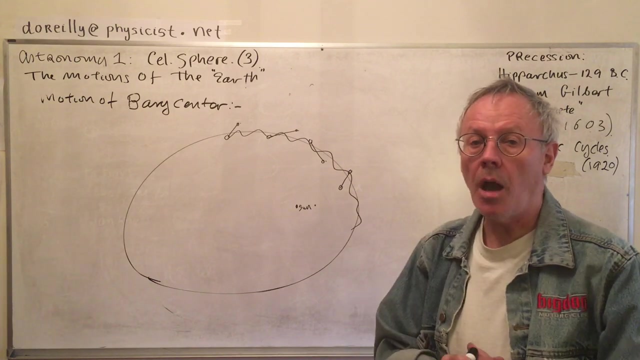 The barycenter follows the orbital path which is the ellipse, But the Earth is doing this. As you can see, it has a little amplitude and a period. It has another cyclical motion. All of these things complicate where we are going to have to look. 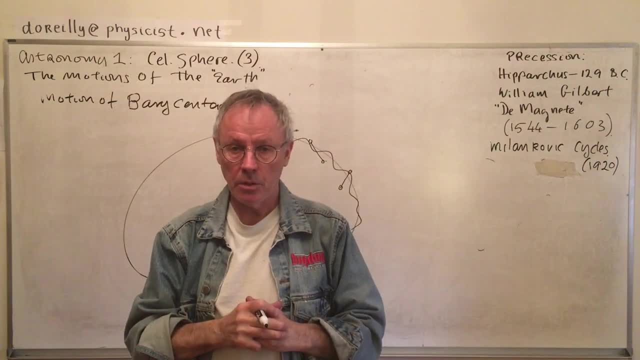 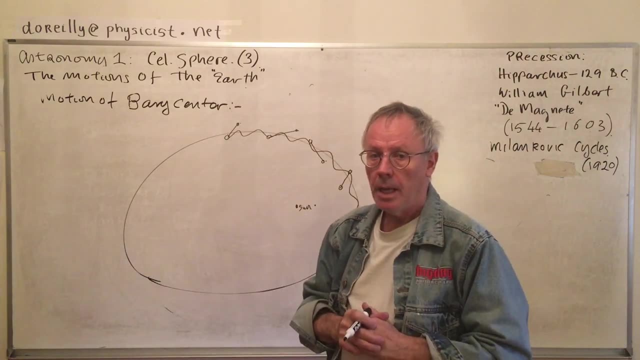 on the celestial sphere, and at what time, to find a particular object, such as a star? Where is it going to be? What are its coordinates going to be relative to the Earth? But these things also complicate time. Now, the last motion is the Milankovitch cycle. 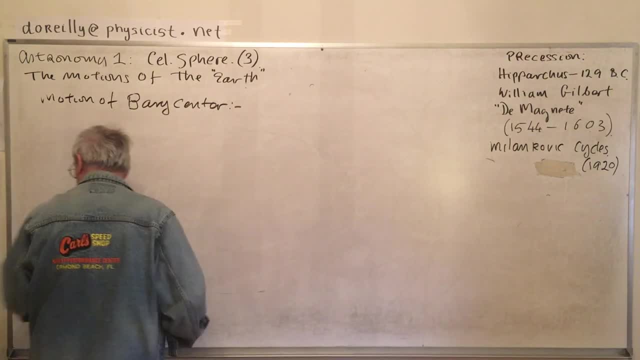 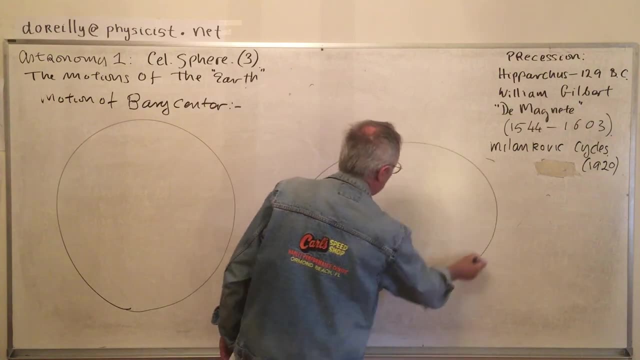 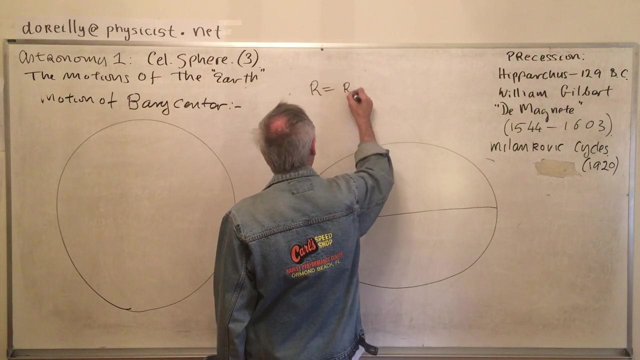 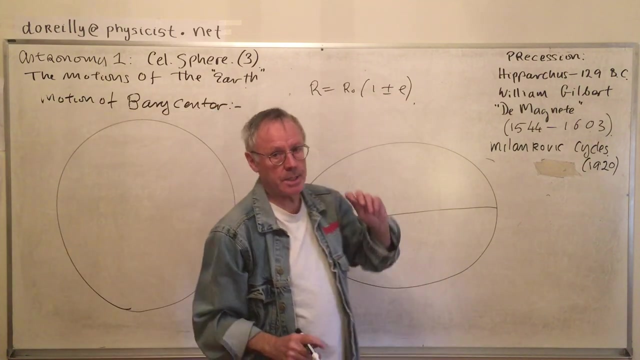 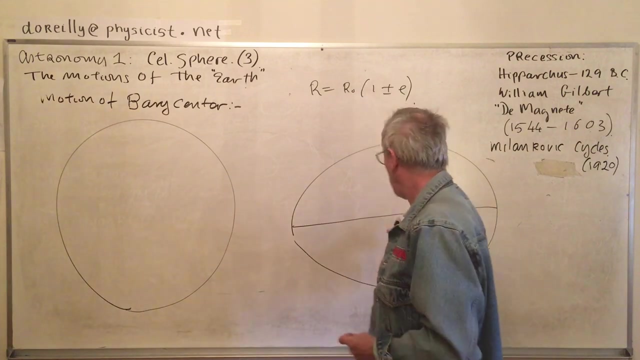 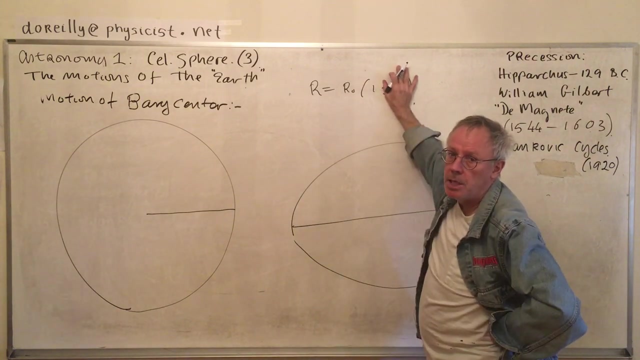 Now, if we take the eccentricity of the Earth, we could write a little equation and say that the actual orbital motion, the radius of the Earth's orbit, the average one averaged out, is circular if this eccentricity is zero. But if we make this a bigger factor or a smaller factor, positive or negative, we 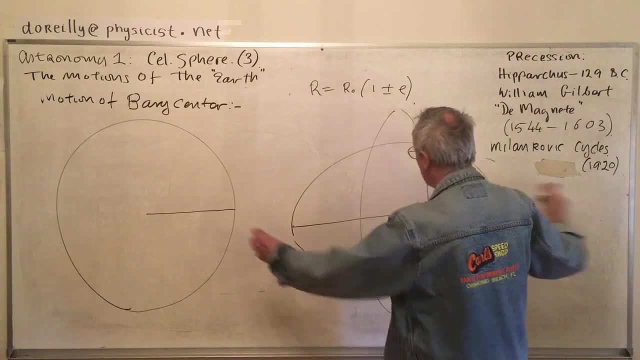 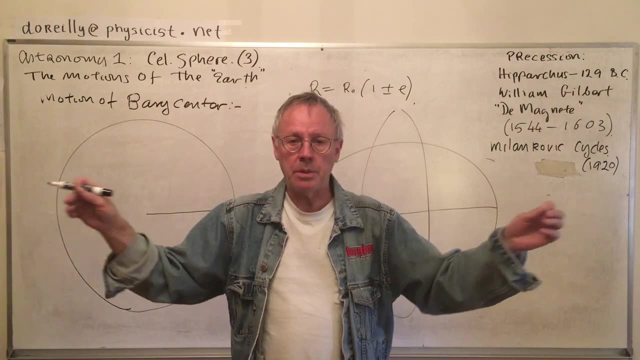 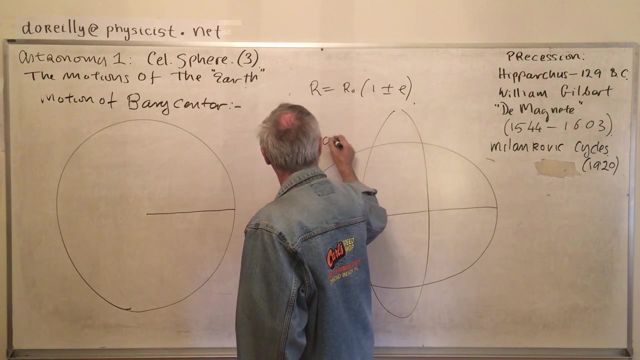 can change the eccentricity up or down, like this or like this, a wobble, so that the Earth's orbit is going from ellipse to circle to different ellipse to circle, to ellipse to circle over a period of 100,000 years. It's yet another periodic. 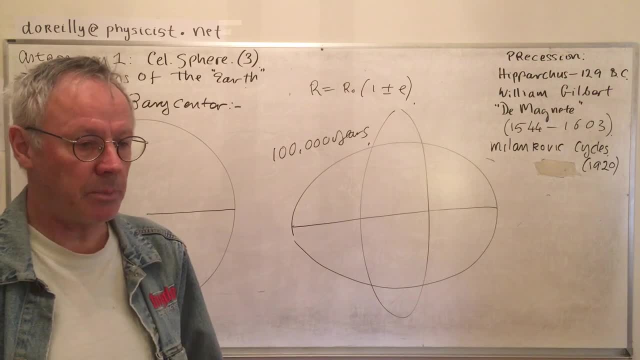 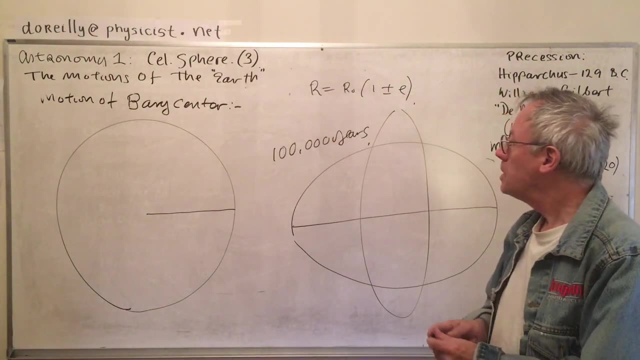 motion. Now there was one other motion of the Earth that I talked about when I did this talk first, and I can't remember what it was because I had seven. I know that, But this is good for now, So let's see what we can do now with regard to 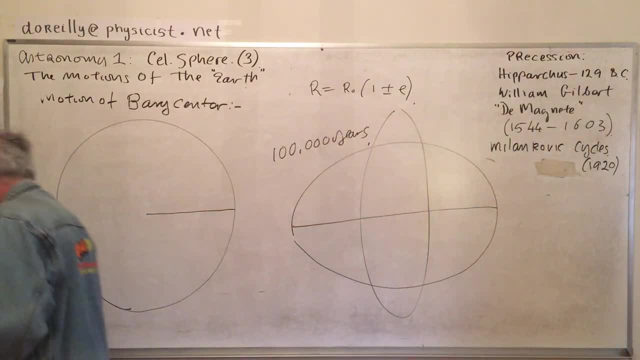 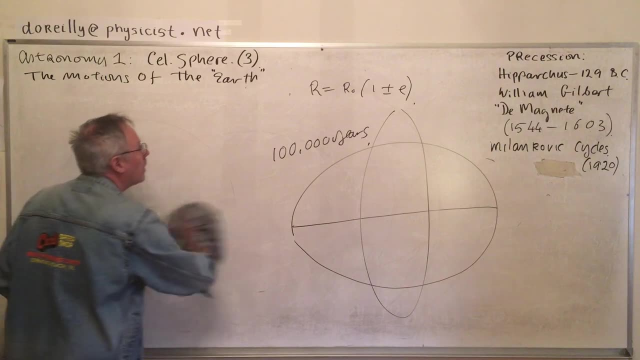 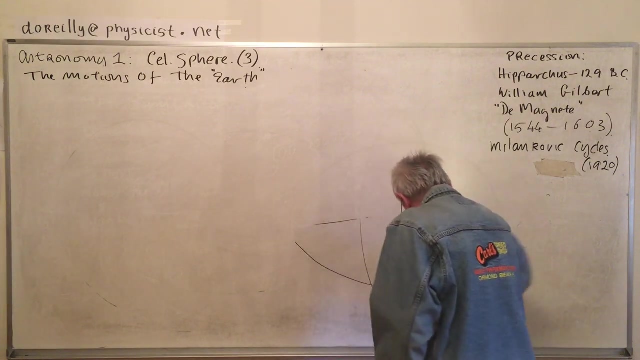 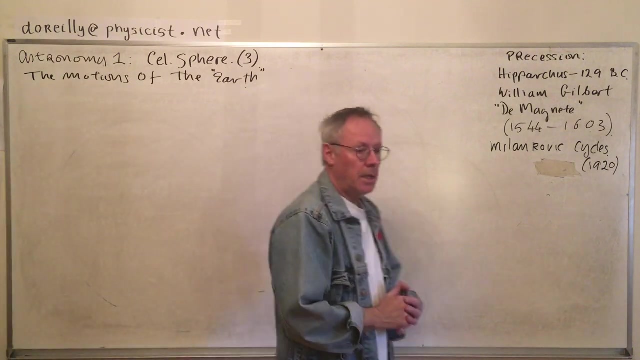 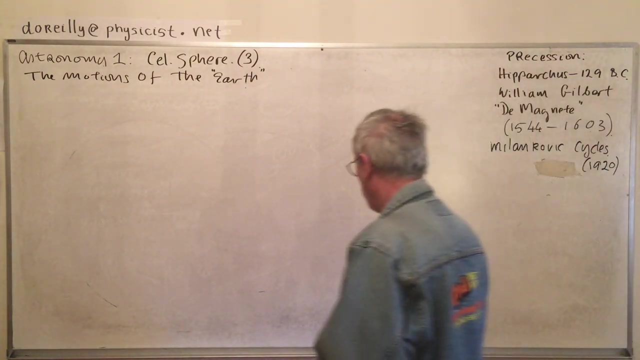 time, sidereal time. Actually, let's not do time. Let's stick with the coordinates. I said I'd look at other coordinates- Right extension and declination. let's call them equatorial coordinates. Let's do a different coordinate system. 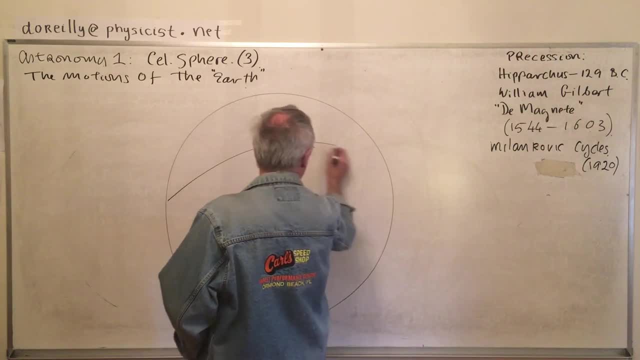 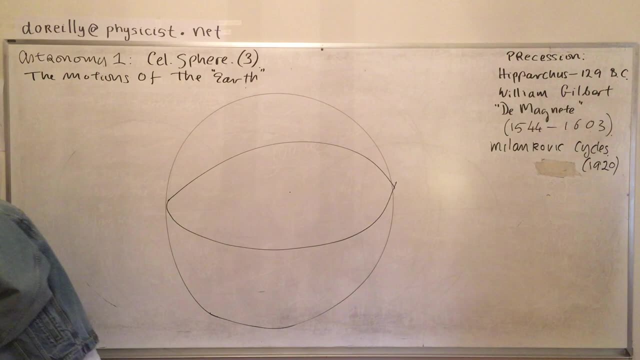 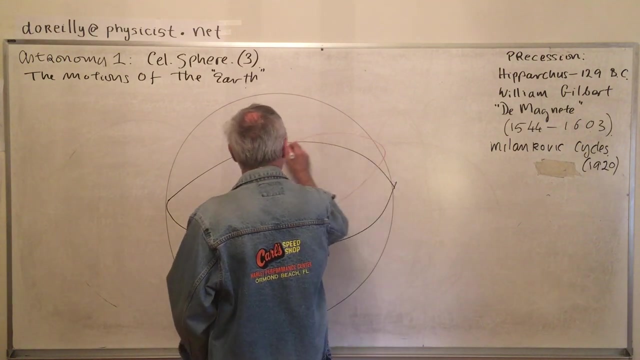 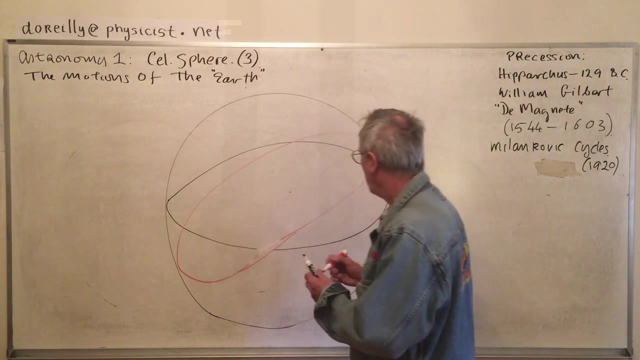 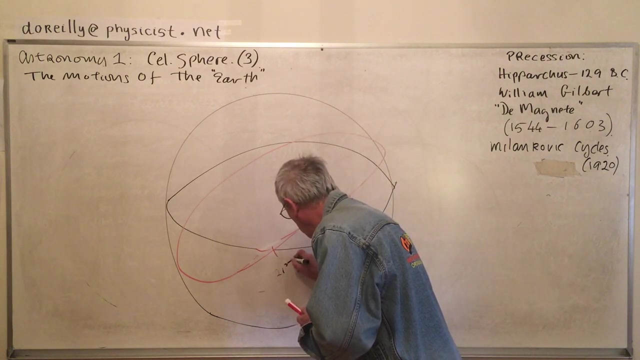 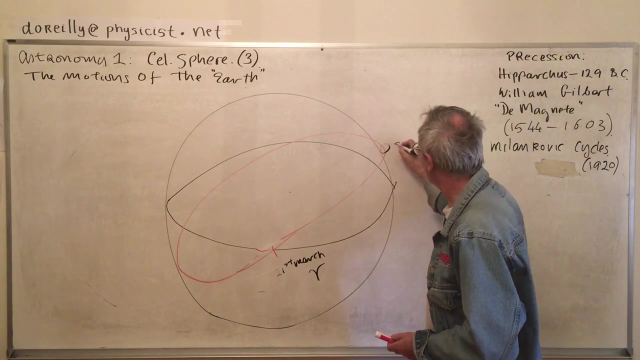 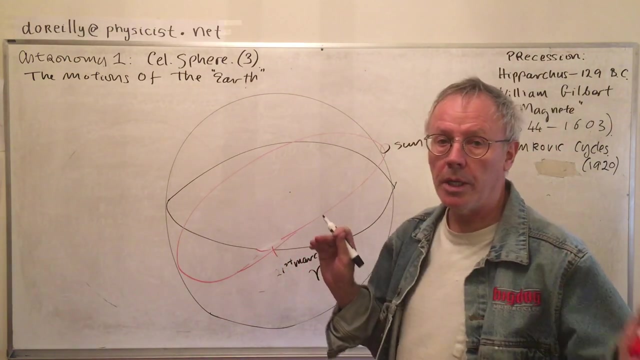 Now I'm sorry I'm not doing the best circles for you guys, because when I put them on the board I don't have time to correct them. Now, this red circle is the path of the Sun across the night sky. the sun, The sun, will move on that path. I don't mean per day, I mean throughout the whole year. 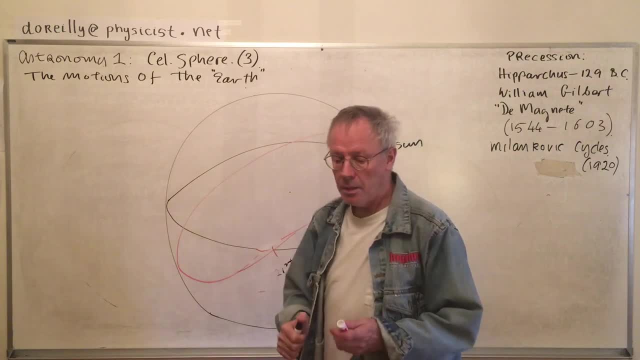 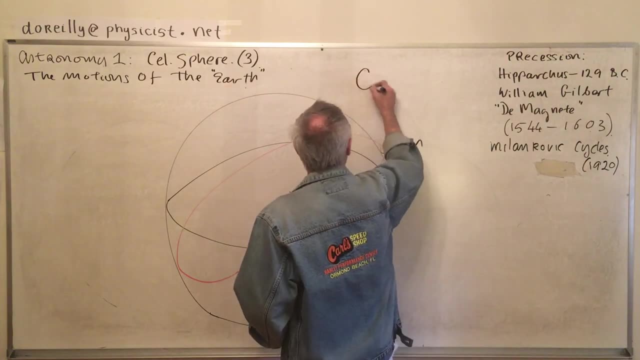 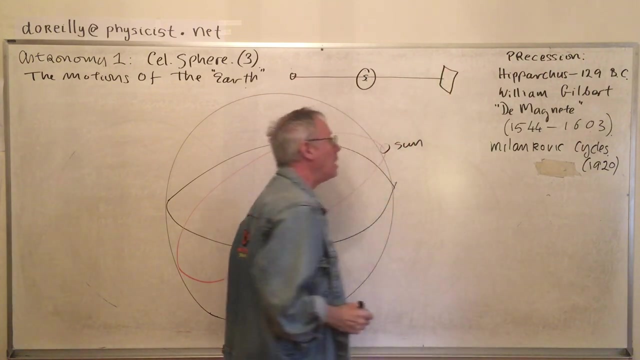 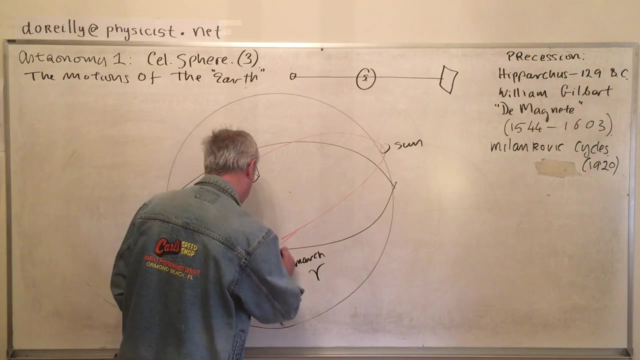 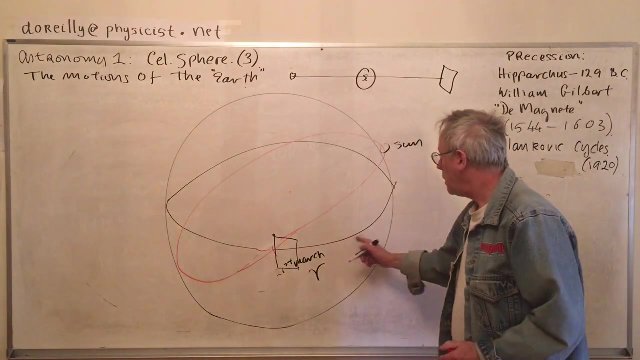 It appears in a different place on the cycle and actually, specifically, it appears in a different constellation. Now, if you were looking at the sun from the earth and on the far side, you're in the constellation Aries- Aries down here, that's the ram symbol. That would be the beginning of the counting of right ascension. 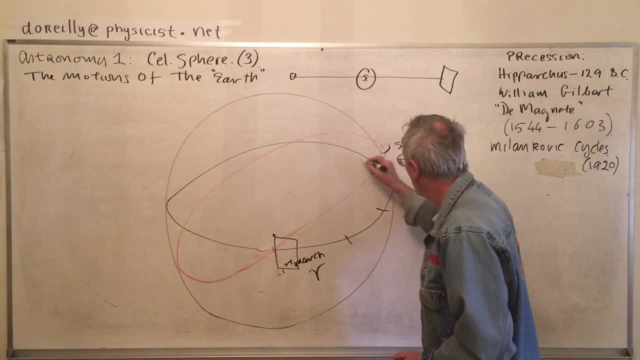 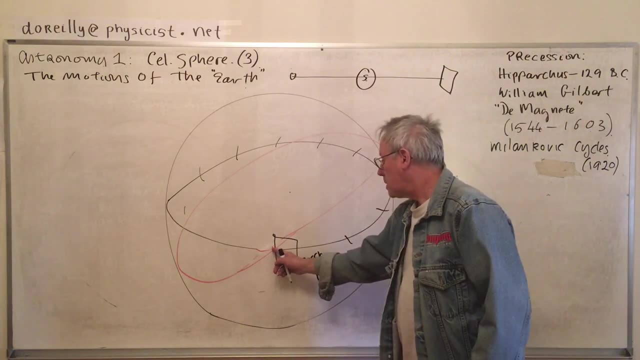 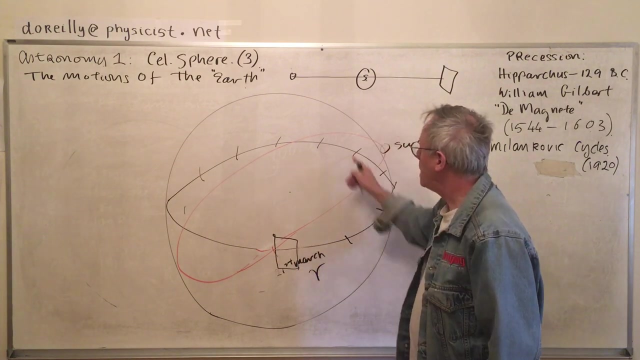 And right ascension is an angle based on this equator, hence equatorial coordinates. Now, unfortunately, what happens is this guy- what we already said- precesses around the place. It precesses over a period of 27 years, so it's moving. 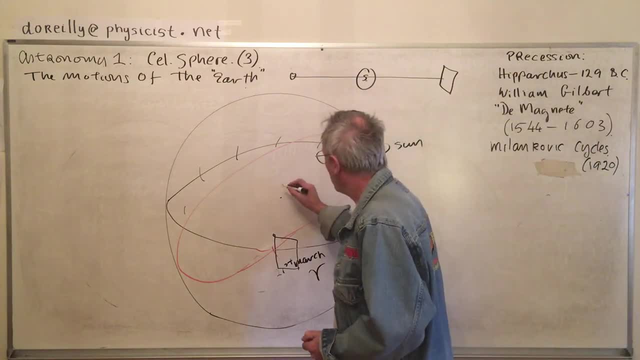 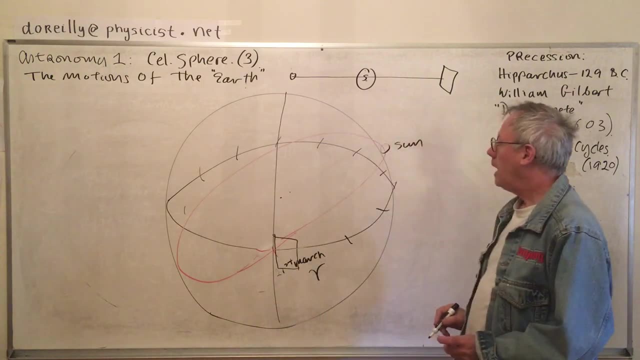 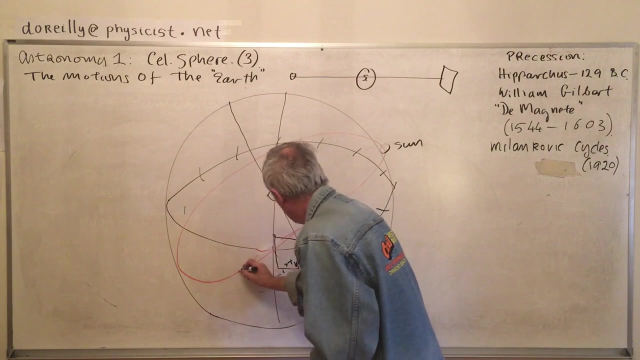 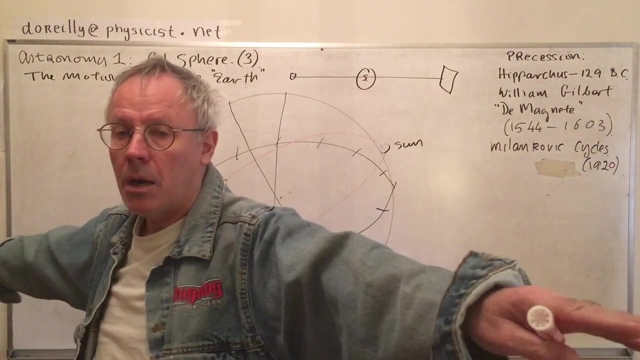 So another way to counteract this problem is: don't set up our coordinate system with poles, north and south equatorially. Choose the ecliptic. Choose the ecliptic as the centre, so that the constellations of our zodiac now lie on what is our celestial equator. 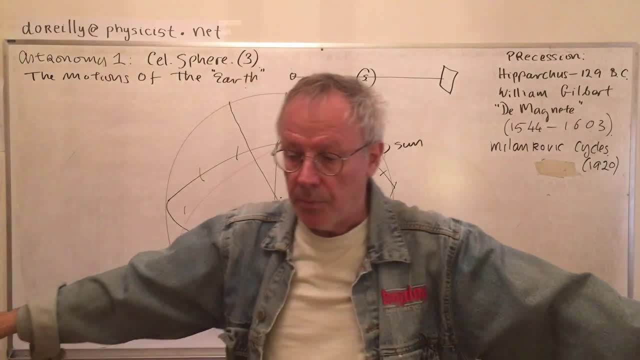 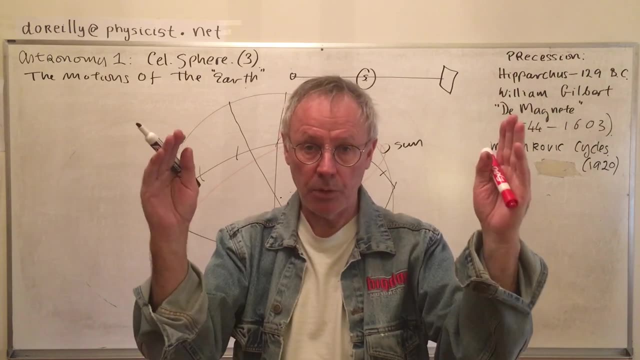 The zodiac. yeah, I don't remember all their names, but there's 12 of them and they take up one twelfth of a circle, That's 30 degrees each constellation. right. Forget the idea of the names of the constellations and just be a scientist. 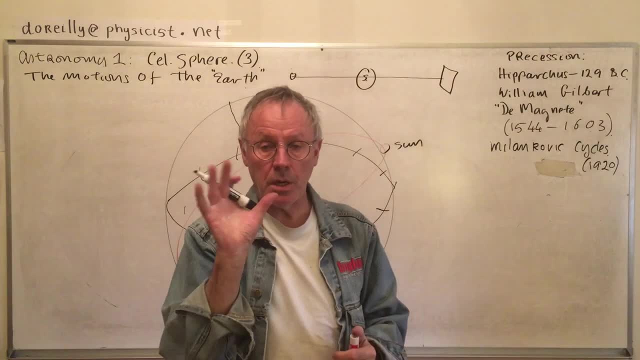 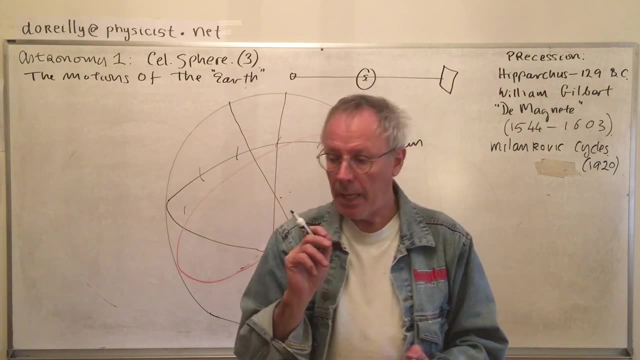 They're boxes. They're boxes on the celestial sphere of a certain width- 30 degrees- And each one of those 30 degree boxes corresponds to an hour, and there are 12 of them. Well then, I guess that's wrong. 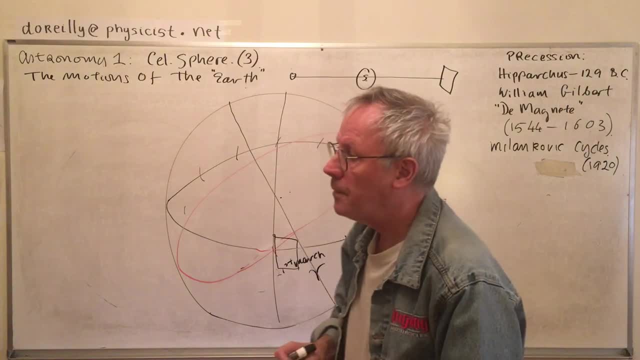 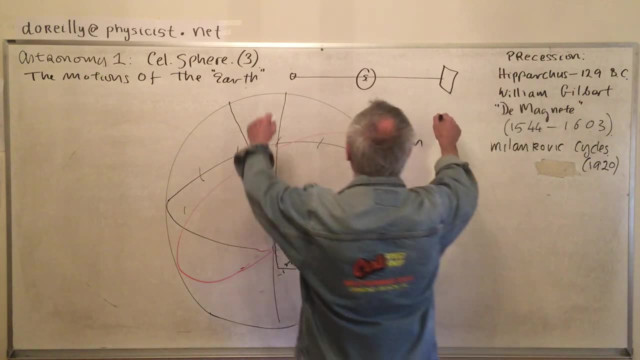 It must be two hours. Whatever, There are 12 constellations in the zodiac. Am I saying this the wrong way? I'll come back to it. Anyway, one way or another, if your sun is blotting out a particular constellation- and it can blot out all of them- 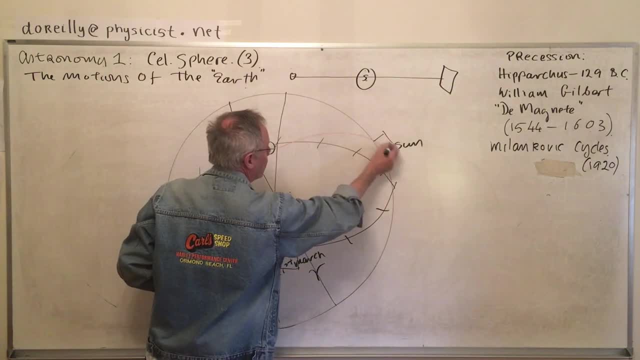 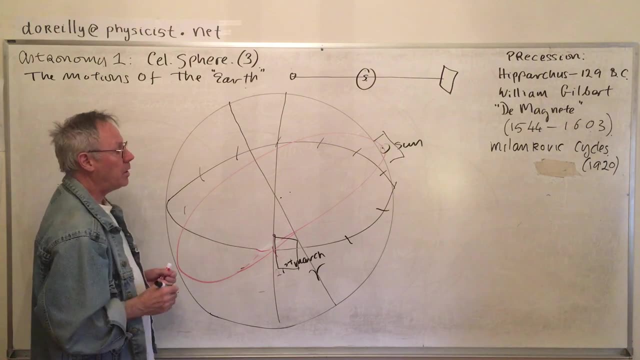 suppose the sun is in the way and you can't see Aries or whatever it is there, then that constitutes like the star sign Aries, The sun is in Aries, and so on and so forth. Now we're in Aries. 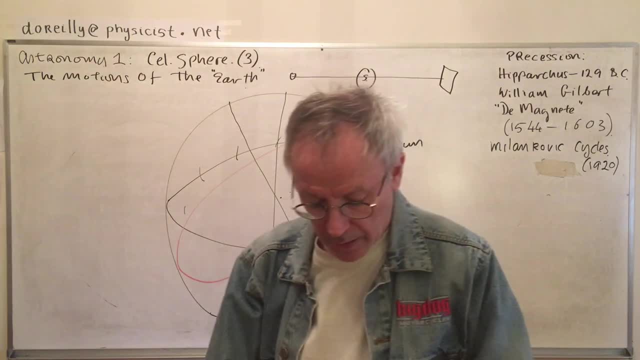 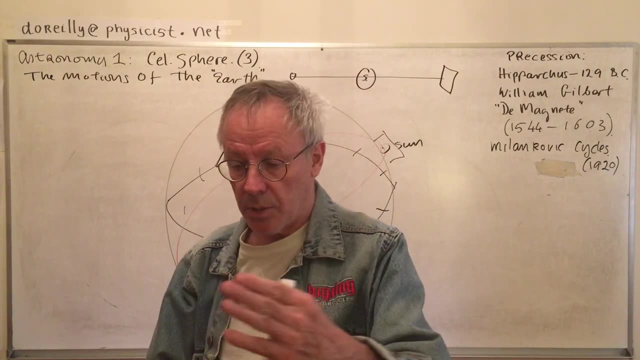 I think we're going into the age of Aquarius. the hippie song That's coming up in, I think 2200 or something. You can look it up on the web. But we're moving into the age of Aquarius out of whatever we're in now. I don't know. 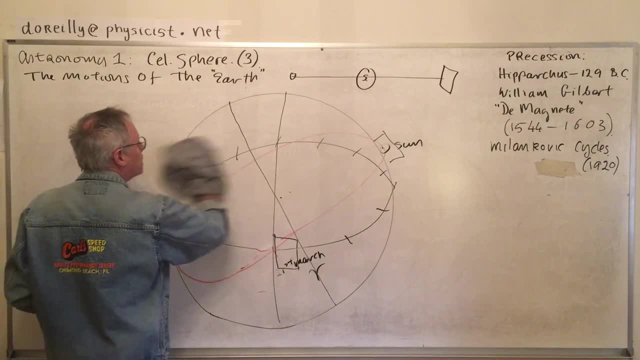 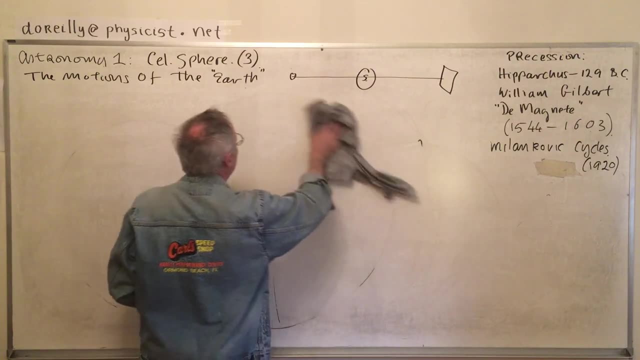 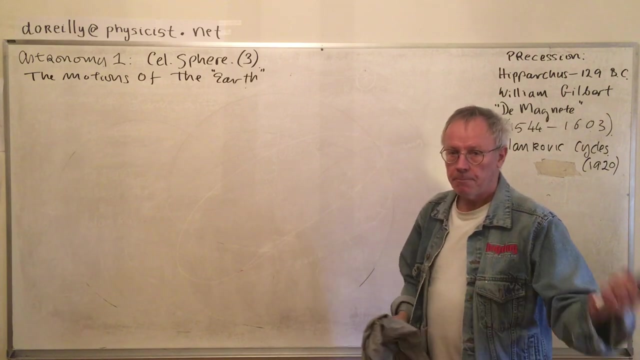 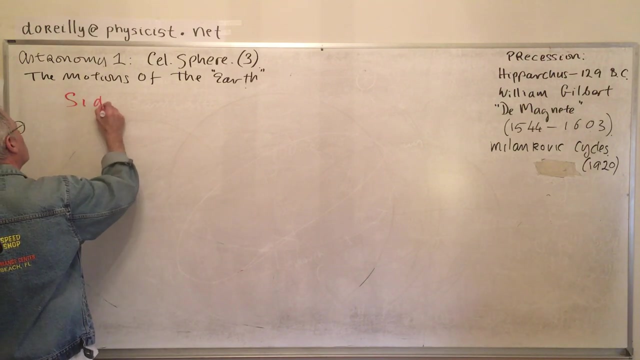 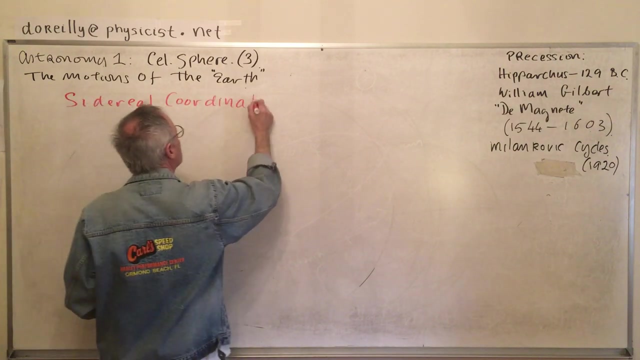 I haven't written down some, But the coordinates that I like are these ones. These are the best coordinates And people don't use them Because even ecliptic coordinates have this precession going on in them. Sidereal coordinates, Sidereal coordinates, I like. 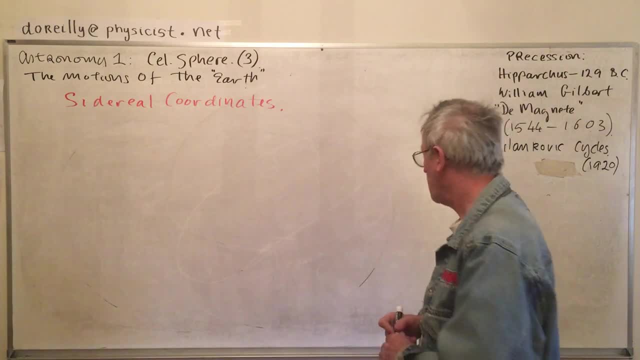 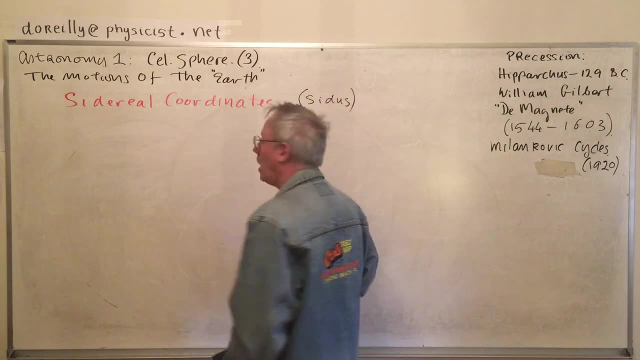 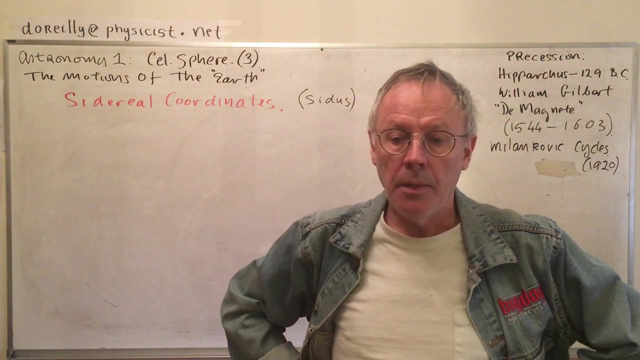 I like them a lot. I think they're nice. Bruce for Scythe. You hear a lot of sidereal things. Sidus, Star- Latin word for star. Anything sidereal is based on the stars. This coordinate system doesn't care if the Earth is there or not. 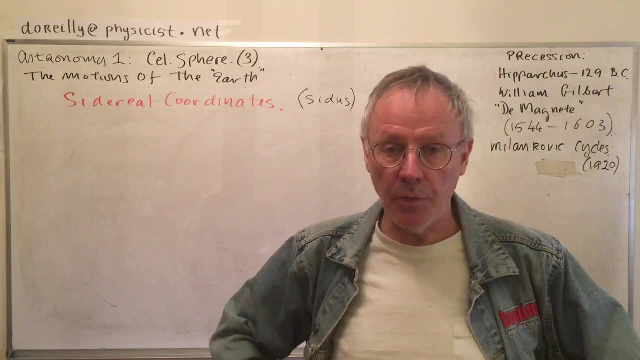 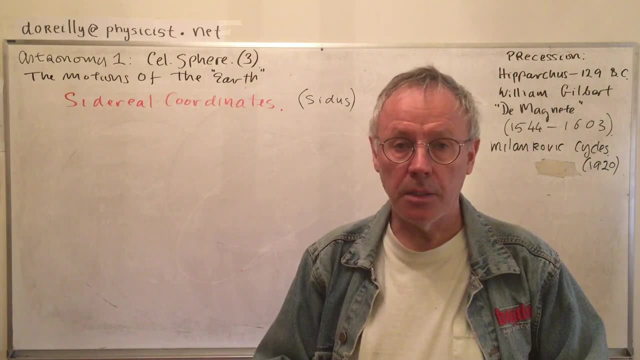 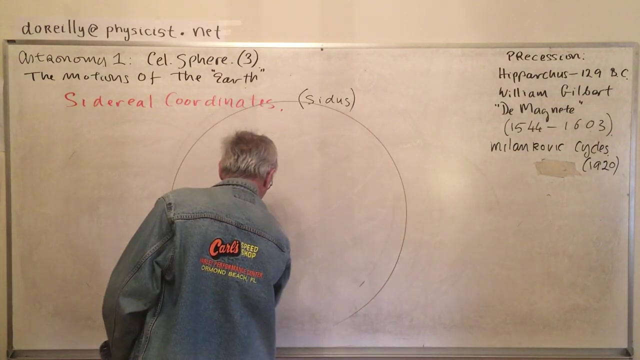 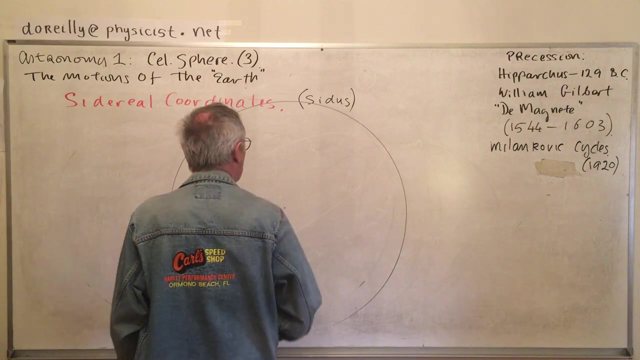 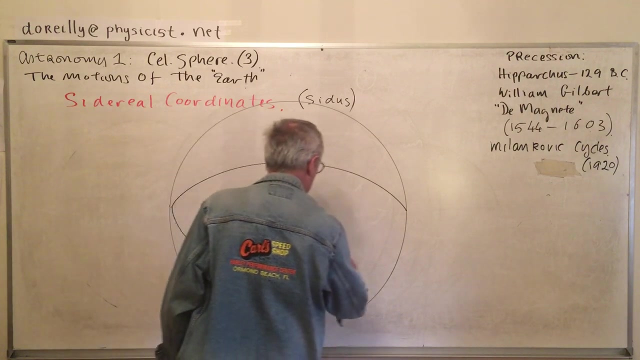 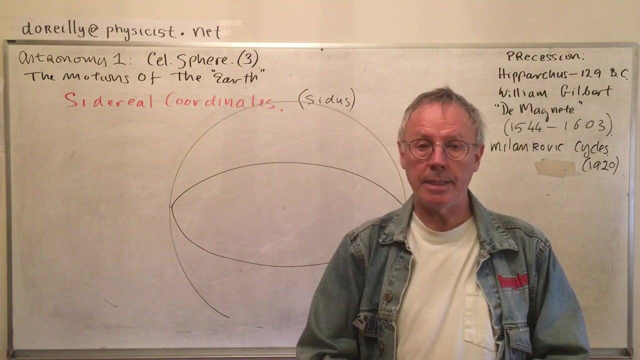 Or the sun. It's just well, assuming we pick our position where the Earth is. This coordinate system has on it just the fixed stars. Now, in the ecliptic coordinate system, they still chose the vernal equinox to be the origin. 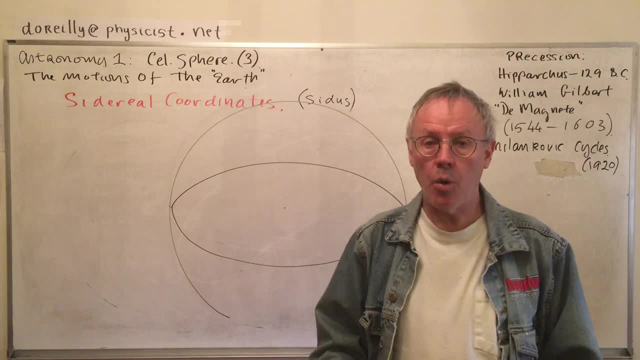 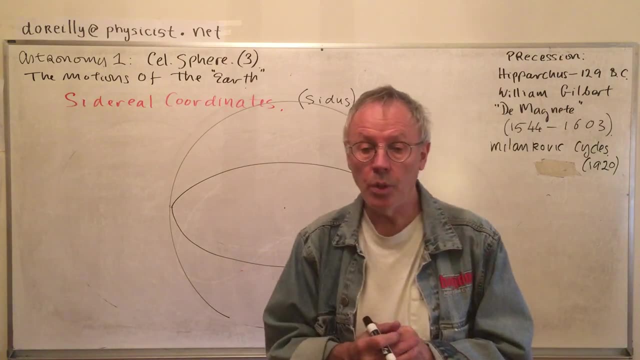 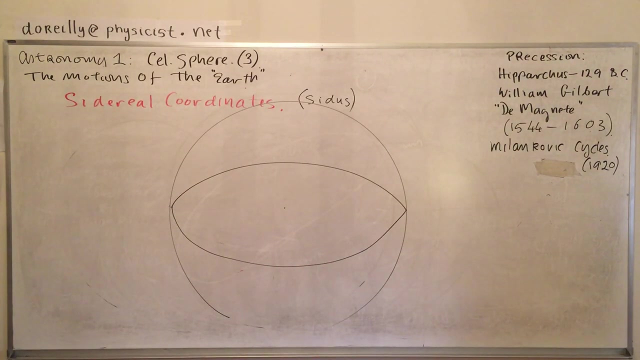 And that's moving right. But in sidereal coordinates you take a fixed star. Now, one star in Virgo according to one guy is a good choice. Let me see who that guy is. Okay, I'm no good with notes. 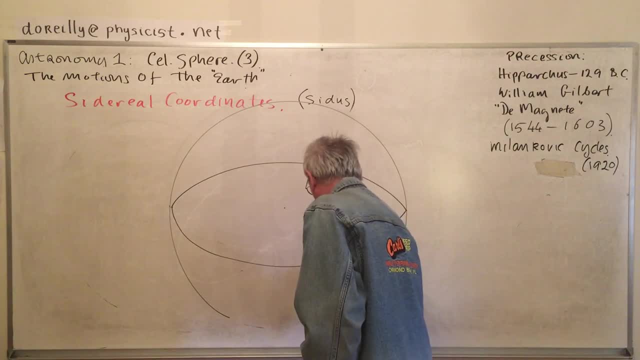 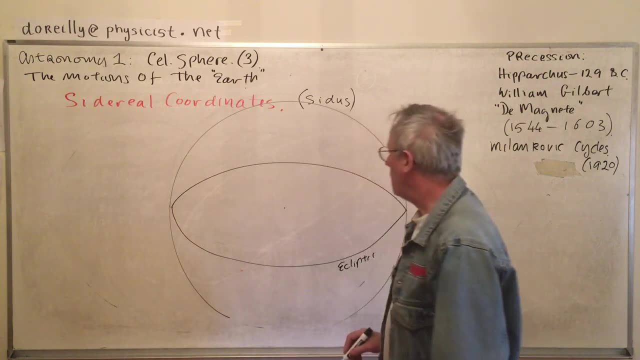 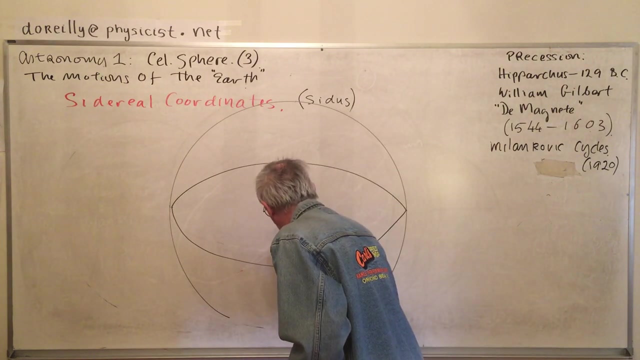 I'm no good with notes today, But if we take the zodiac- This is the ecliptic Right- We forget about the tilt of the Earth or anything, But we just take a star, A star in Virgo- I think it's Pi Virgo. 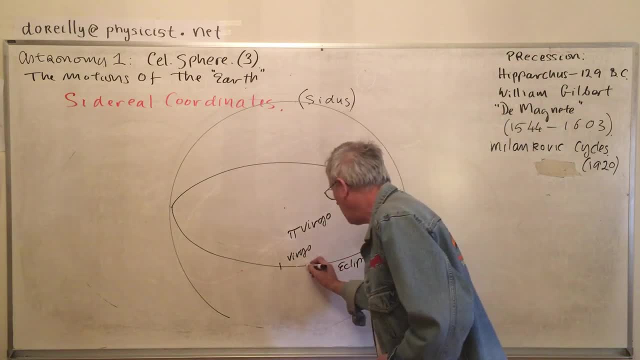 Is the star that some guy suggested we should choose. So that would be the constellation Virgo, And the next constellation, And the next constellation, And the next constellation, And so on and so forth. Let's find those constellations, Okay. so 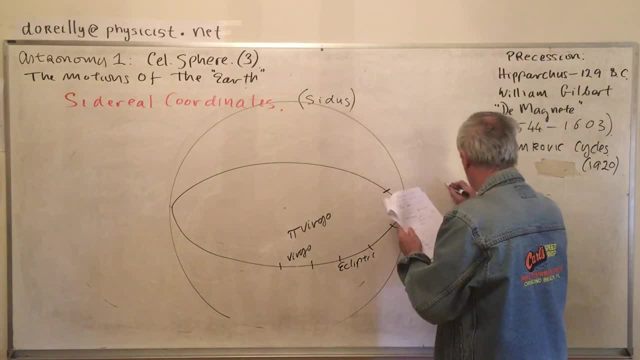 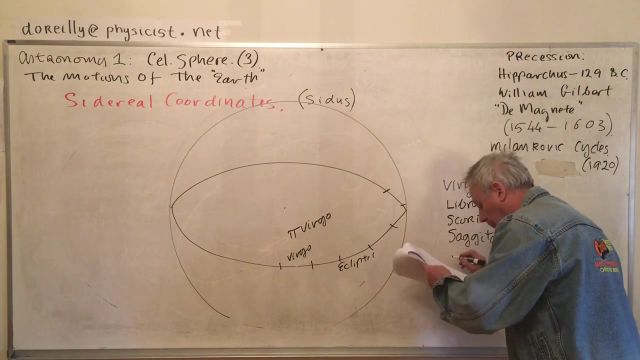 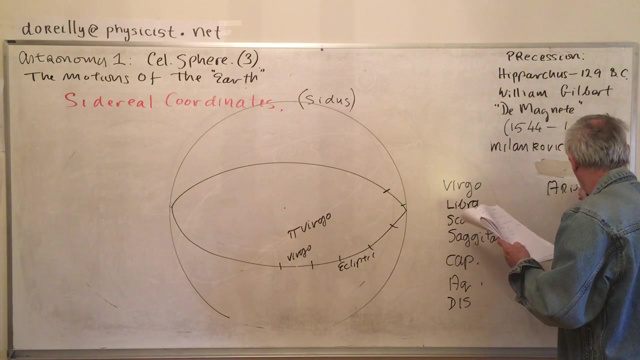 It starts out with Virgo. I do it in abbreviation: Capricorn Aquarius. That means we must be in the age of Capricorn. I don't know what this is. I wrote it in brief: Taurus Gemini. 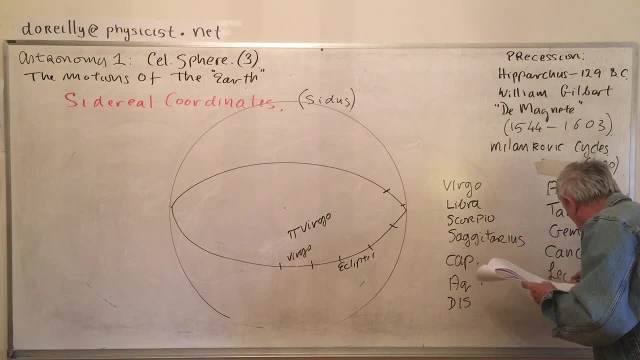 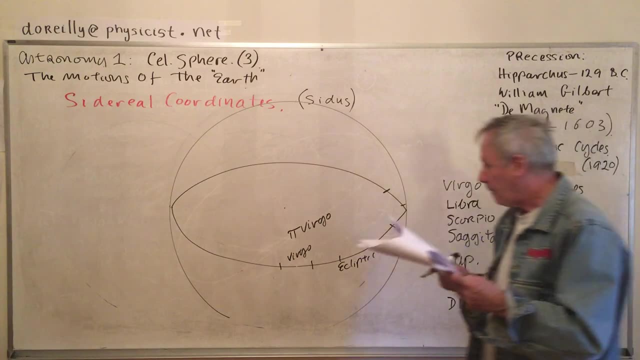 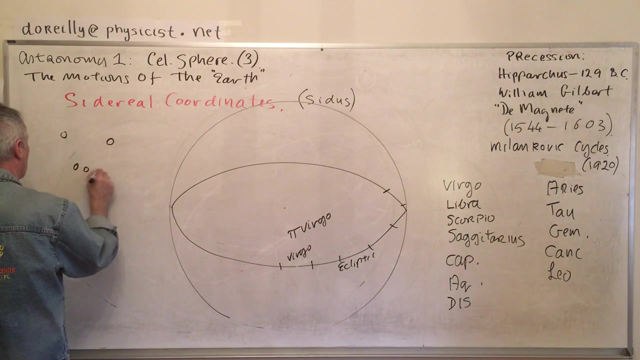 Cancer. One, Two, Three, Four, Five, Six, Seven, Eight, Nine, Ten, Eleven, Twelve. Okay, I got them Now. incidentally, When you label stars in the constellation, you go: Alpha, Beta, Gamma. 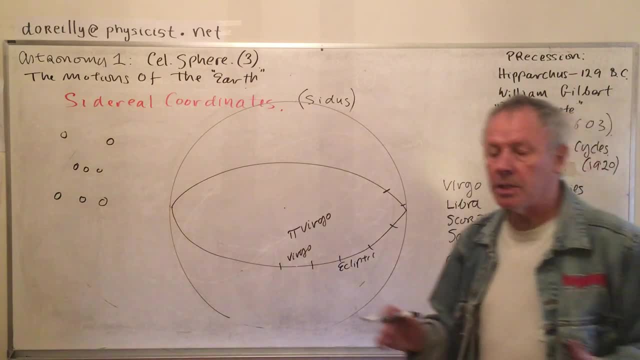 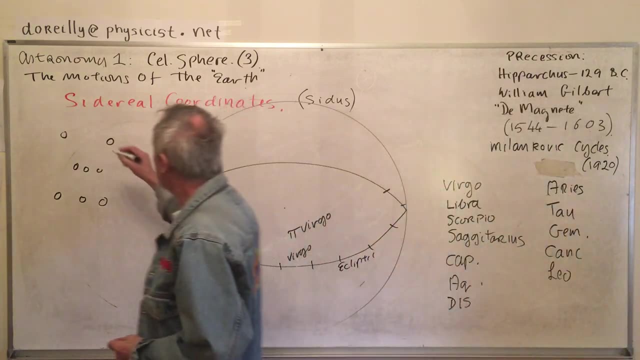 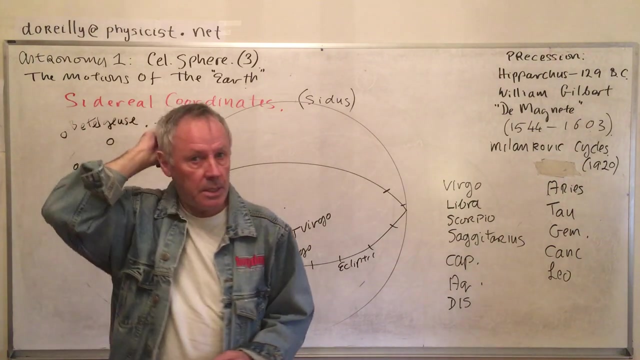 So Pi, Virgo, That's going to be a star that's not that bright in Virgo, That's going to be the brightest star in Virgo. The brightest star in the constellation Orion is Betelgeuse. I don't carry a lot of the names of these stars and constellations around in my head. 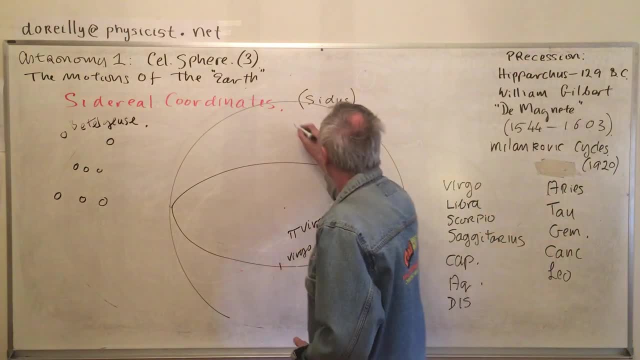 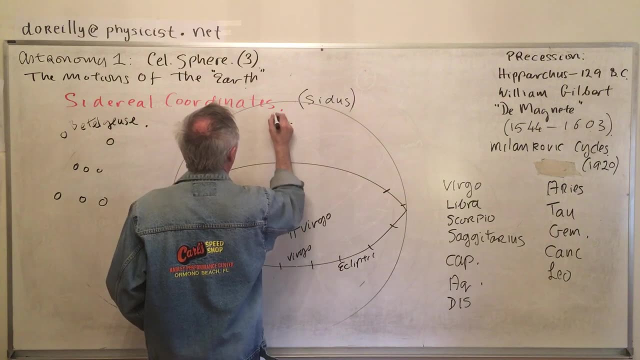 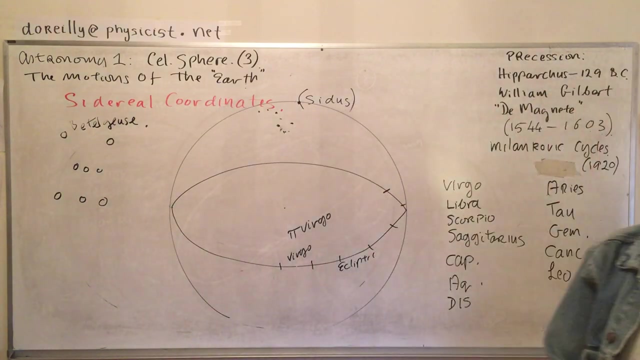 by the way, though, Anyway. so what we do now is we take these stars. They're all fixed. For example, Ursa Major is up here, And these two stars point to Polaris. Polaris is pretty close to being on the axis of this coordinate system, but not exactly. 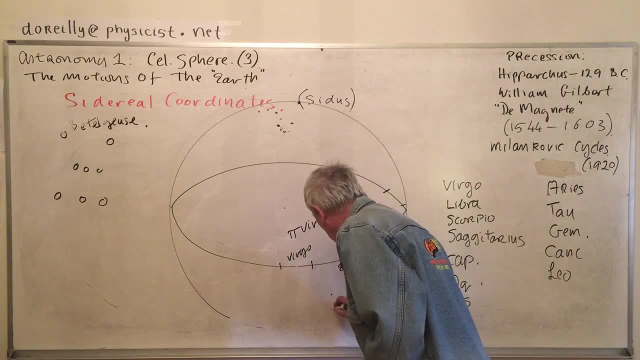 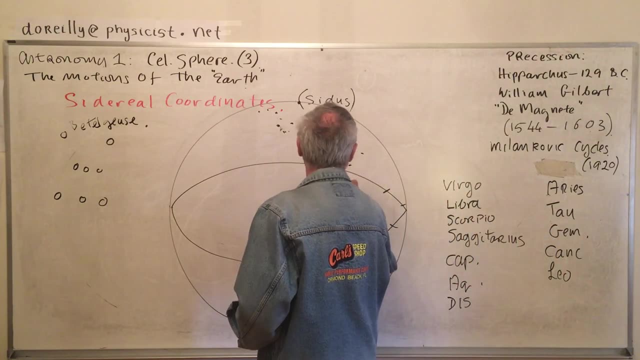 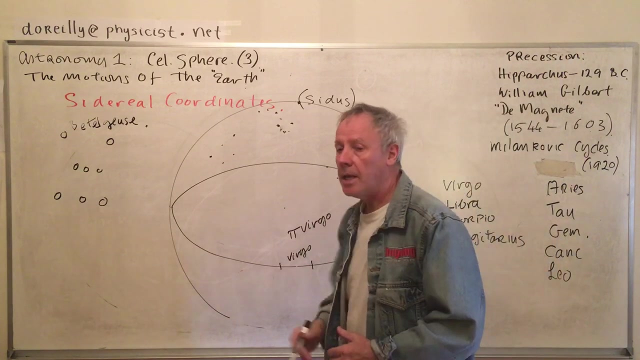 And the Southern Cross is way down here in the Southern Hemisphere, And all the other constellations, Cassiopeia, wherever they are, are fixed And nothing moves. Each one has a particular coordinate It's going to have- Every star is going to have- an angle of, let's say, declination, an altitude. 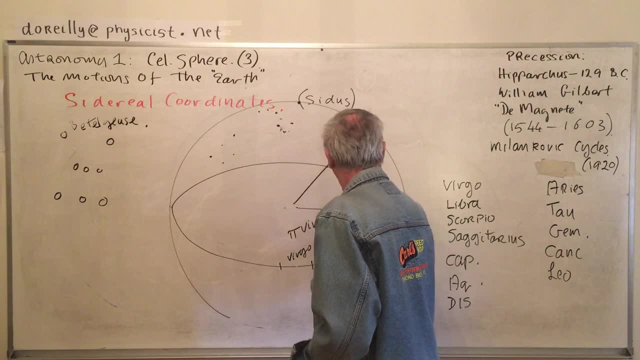 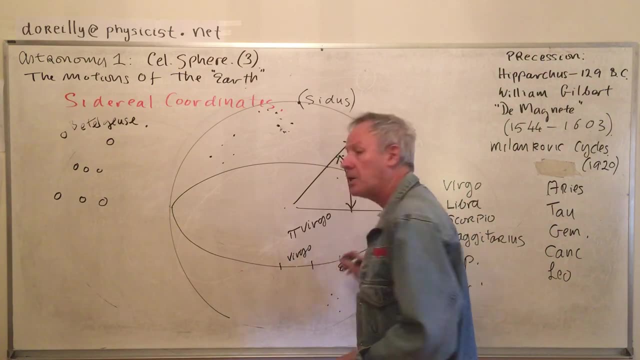 Okay, Which is going to be still a declination, And whatever way you choose to put it in, I like degrees. So this star is going to be, let's say, on this meridian. That's the number of degrees it's got anti-clockwise of Virgo. 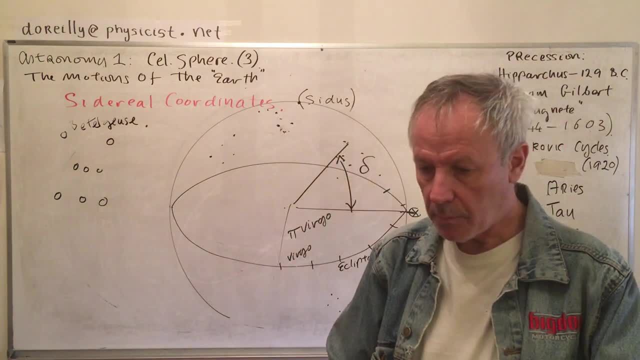 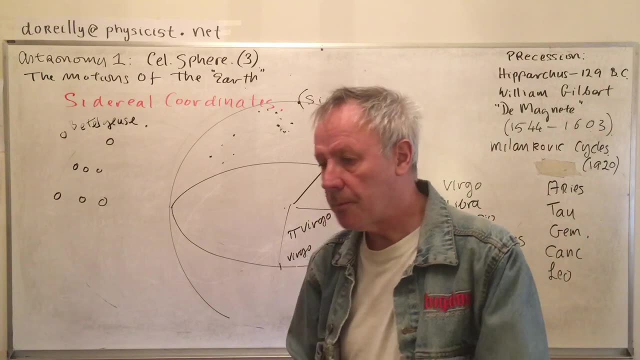 The sidereal coordinate system. Okay, I'm going to stop that talk for now. The next talk will be on time- Sidereal time- Because this is the way it works. When the sun rises and sets, it takes 24 hours to do it. 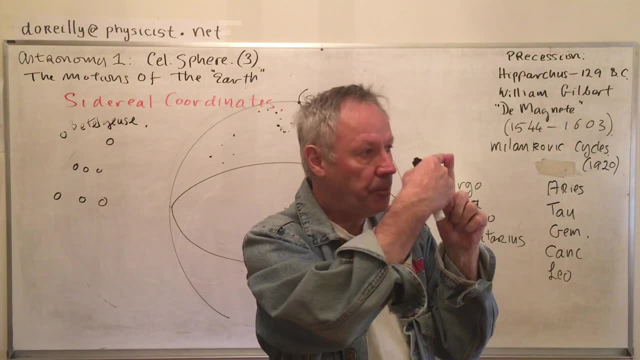 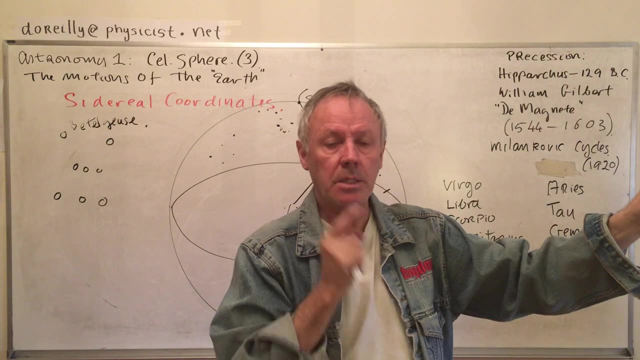 Mark a point on your window And you're in bed And you put a little sight. You need two things to sight And you look out here and you see the sun is on the window. ledge at 6 o'clock in the morning. 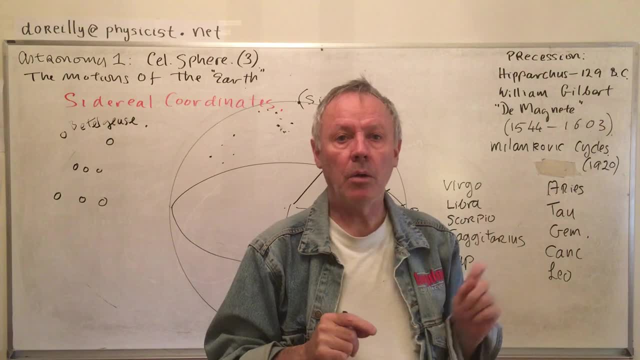 The limb of the sun. That's the edge of it At 6 o'clock Now. when you get up at 6 o'clock the next day, you expect the sun to be right there in the same place, And it will be. 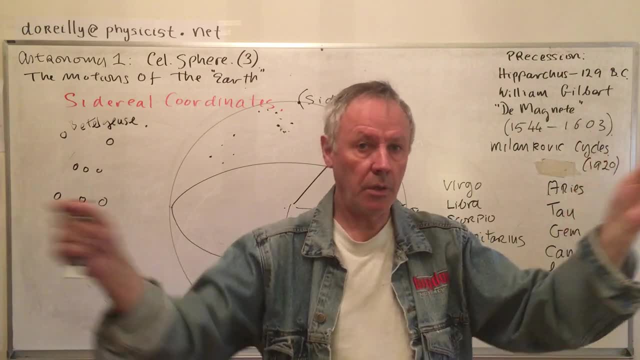 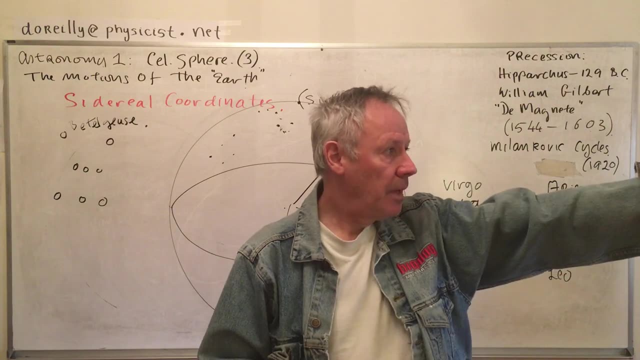 Give or take a couple of little motions due to the other factors, But the rotation of the Earth will be 24 hours. Let's take, we take a star now And we do the same thing. We sight on a star And we wait for it tomorrow night.